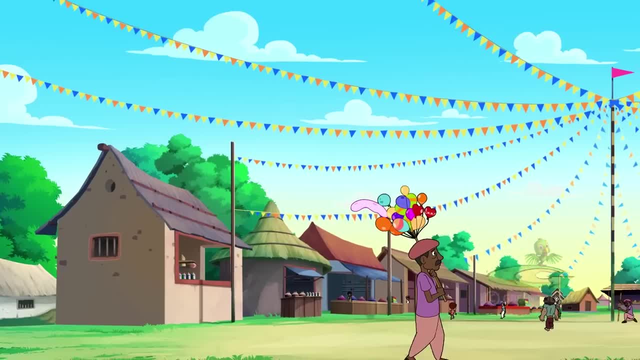 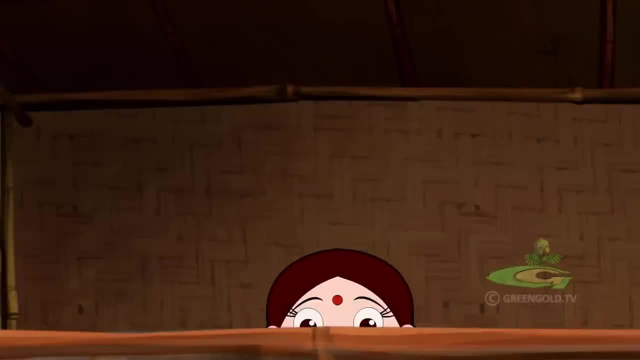 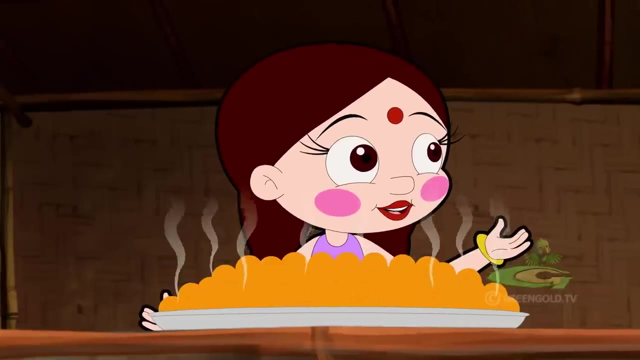 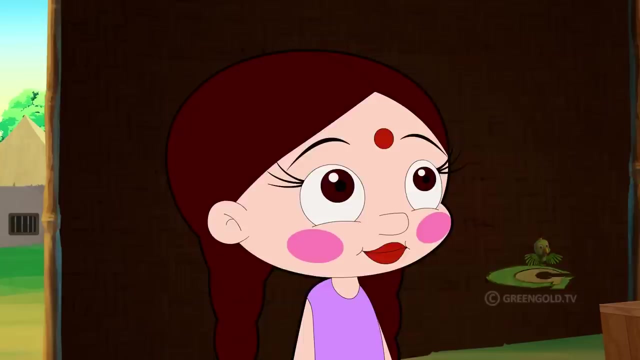 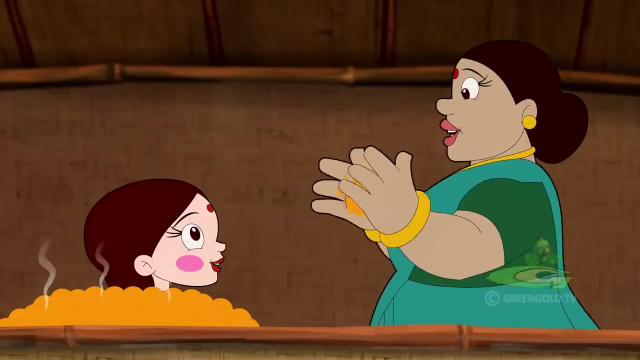 We will welcome the amazing crops of this year with some hot, delicious laddus. Yes, Dholakpur has had such a good harvest after so many years. Yes, A happy occasion like this must be celebrated. But be careful: The children might try to steal the laddus even before you distribute them. 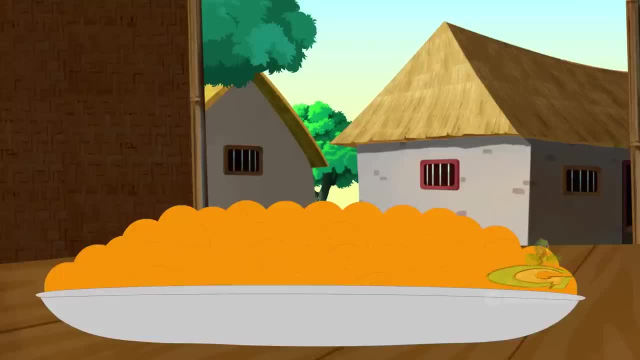 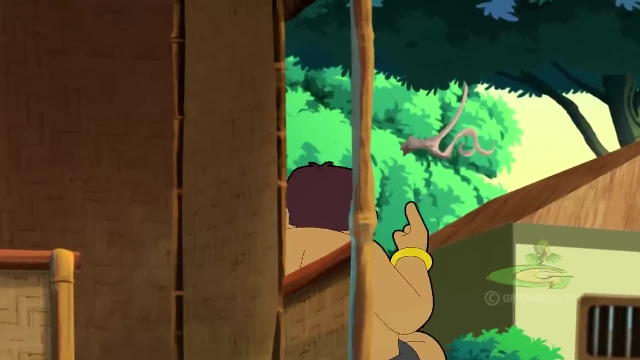 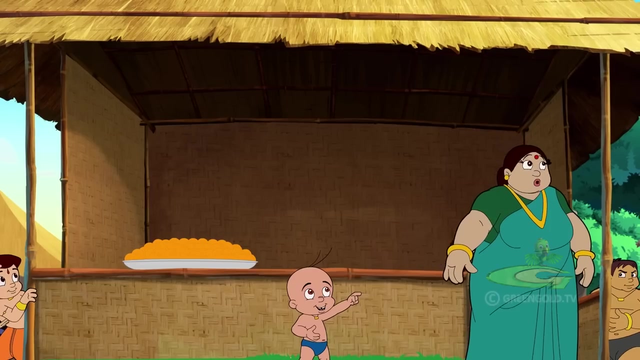 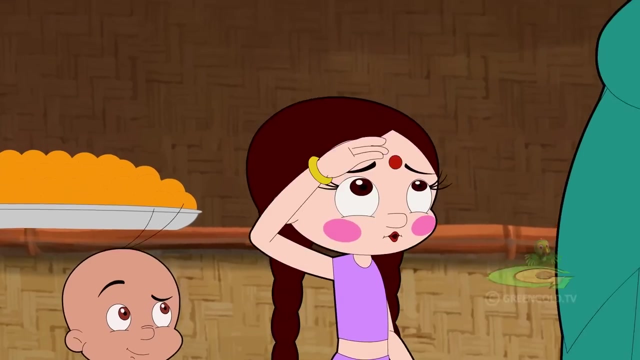 I'll catch her attention and you take the laddus The moment they look somewhere else. we will attack on those delicious laddus. Chutki Mousy, look over there. There's a beautiful kite in the sky. But, Raju, where is the kite? 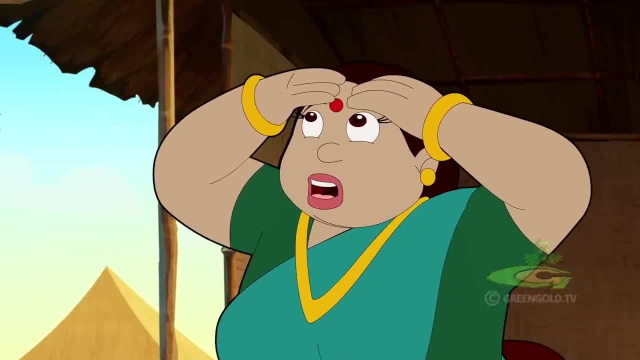 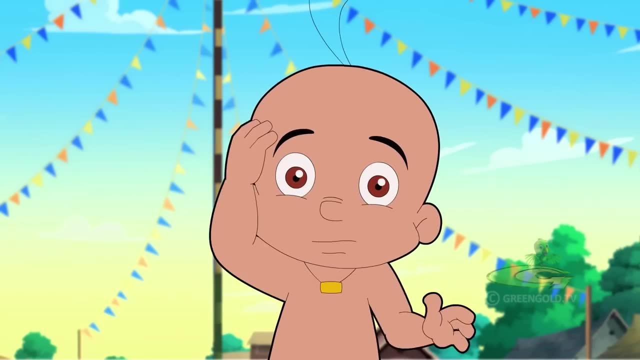 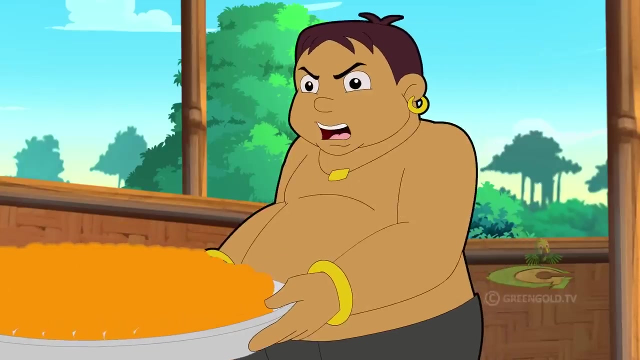 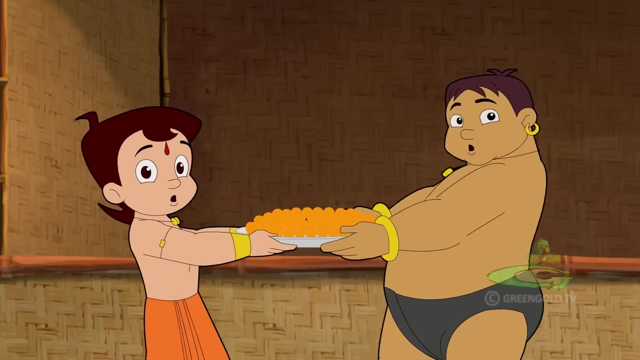 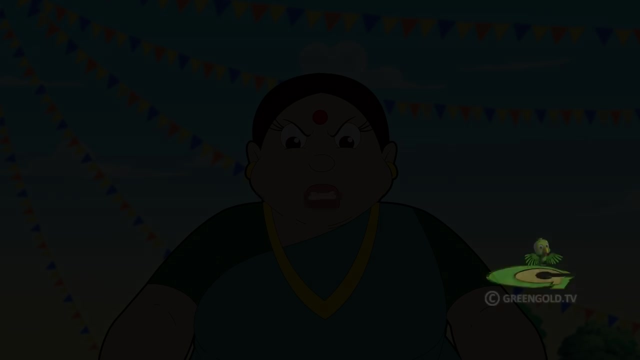 Over there. It's hidden behind the tree. now It'll come out. Wait and watch, Leave Go away. These are mine. When children don't have anything to do, they become really mischievous. Oh no, Our kite doesn't have laddus today, Just hard work. 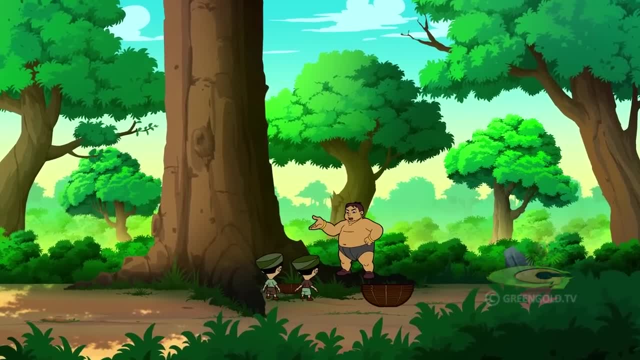 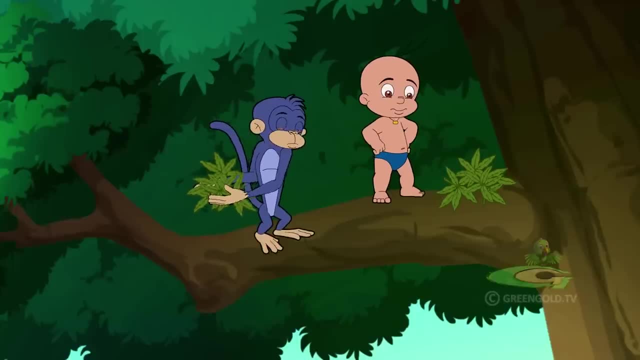 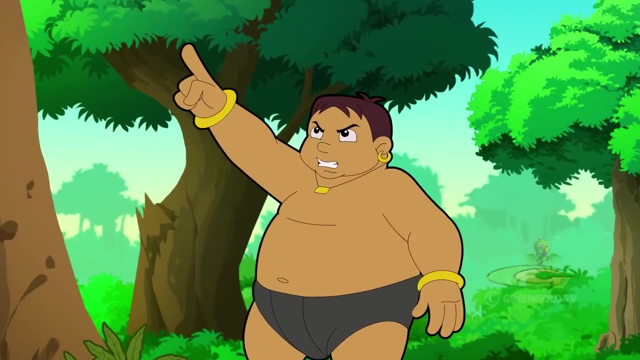 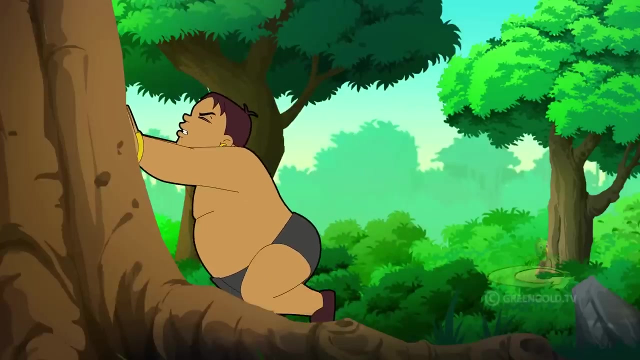 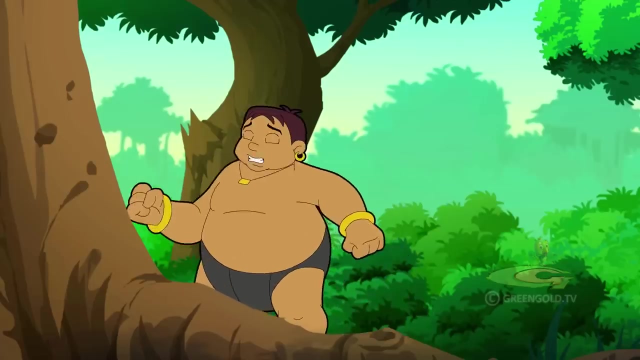 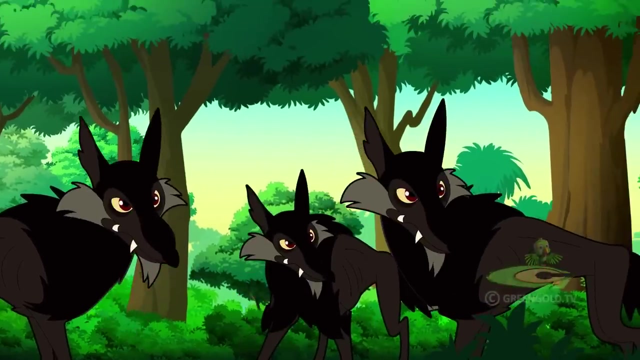 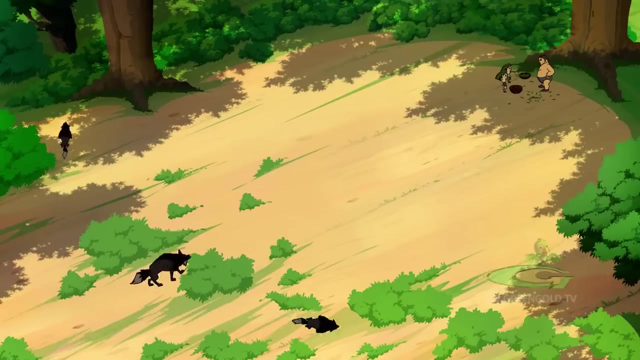 Just hard work. We were just about to get those laddus But Jaggu and Bhim came and spoiled the whole plan. We didn't spoil the plan, You spoiled the plan. I am not going to spare both of you. Oh my God. 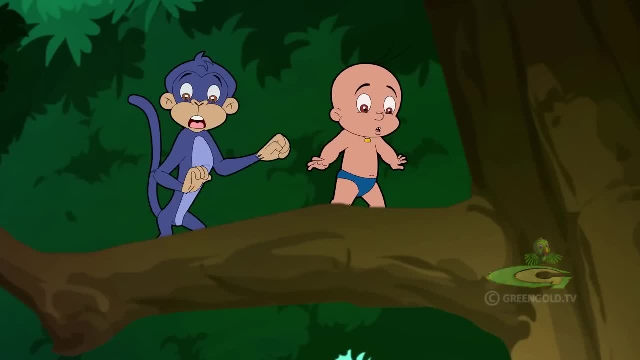 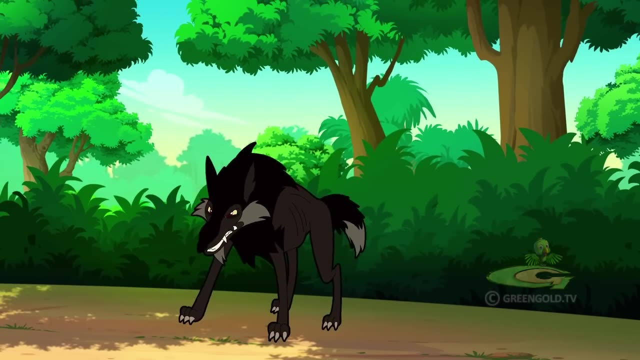 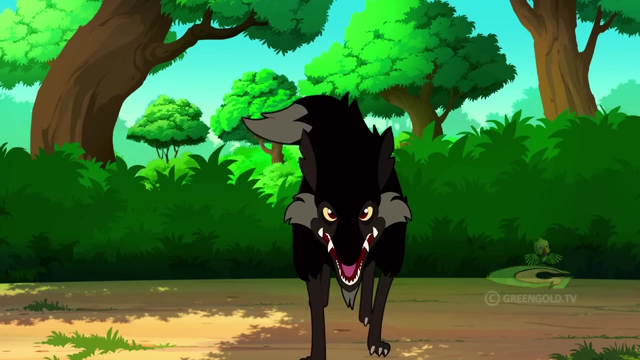 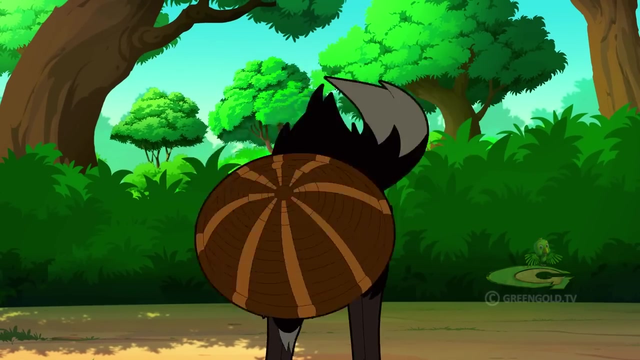 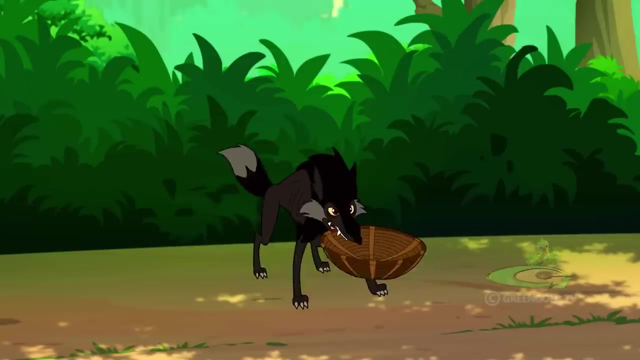 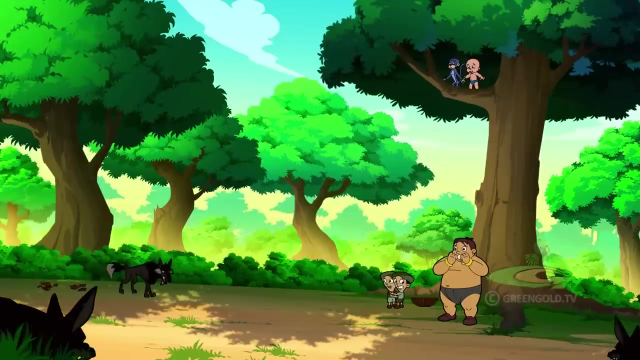 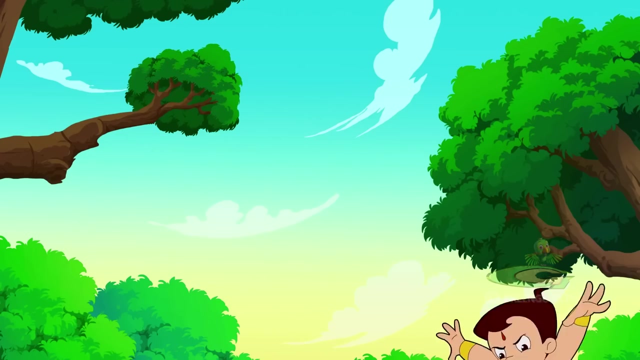 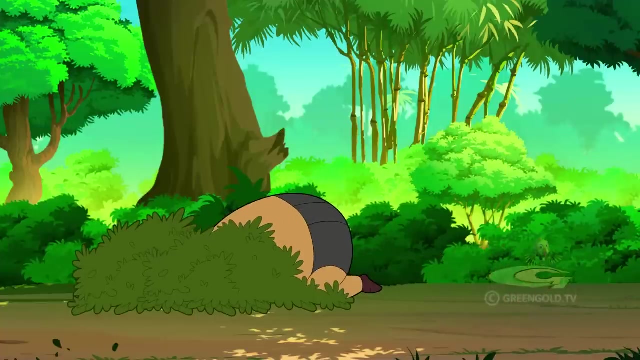 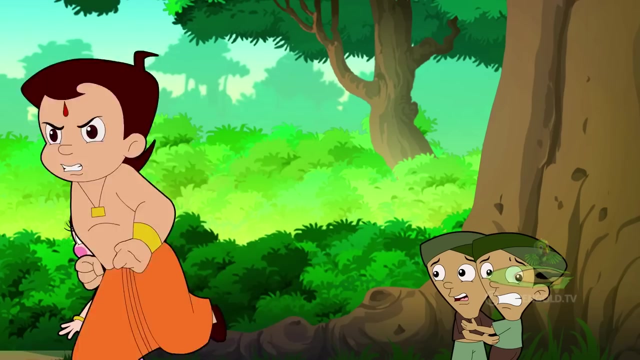 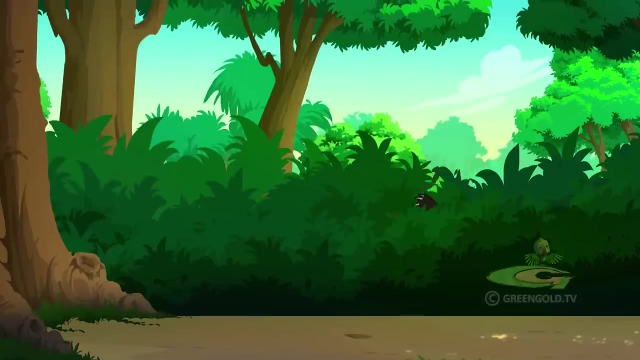 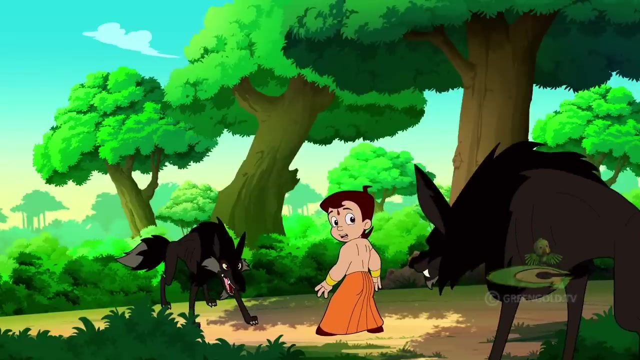 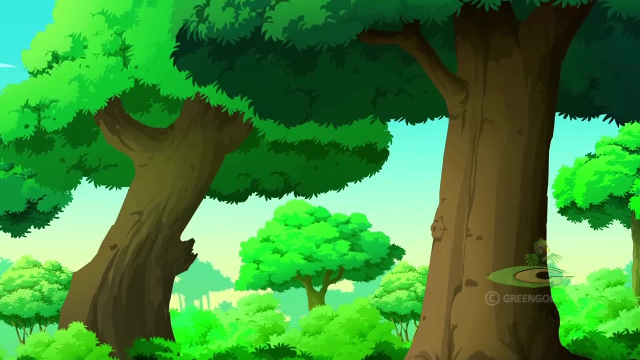 Oh my God, Oh my God, Get back everyone. I am so huge that I am unable to hide behind these teeny tiny bushes. I am so huge that I am unable to hide behind these teeny tiny bushes. I am so huge that I am unable to hide behind these teeny tiny bushes. 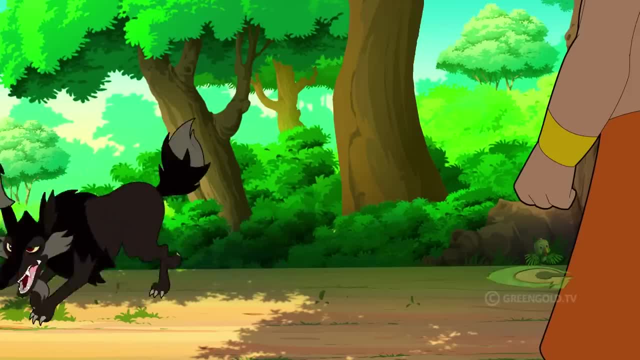 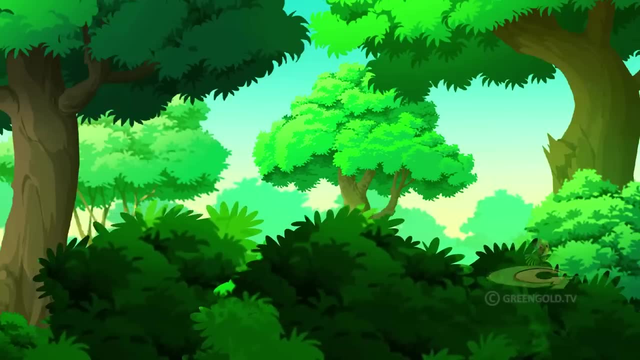 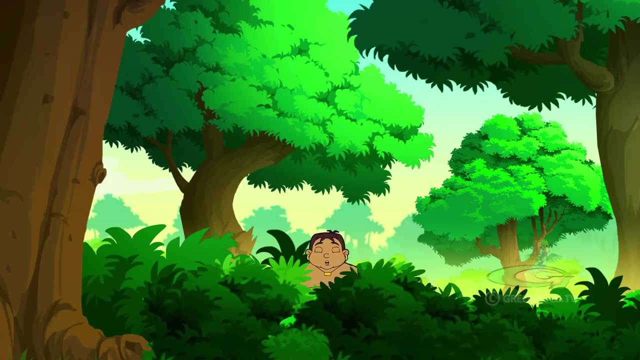 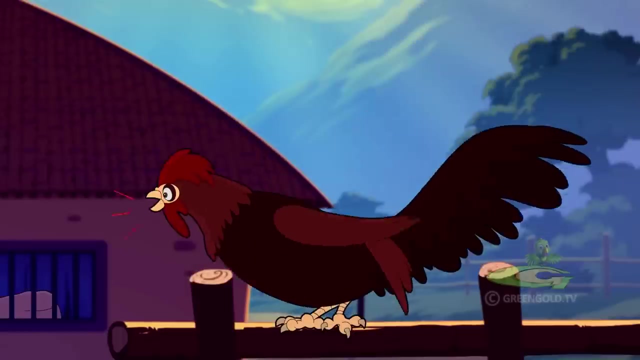 Get out of here, otherwise Yay, Come outside. Kalia, You're scared, but the bushes are shivering. I am not scared. I was just trying to look for a weapon to scare away those wolves. Oh, Please help us. 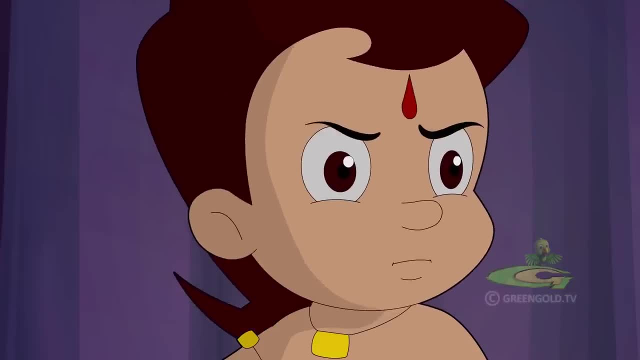 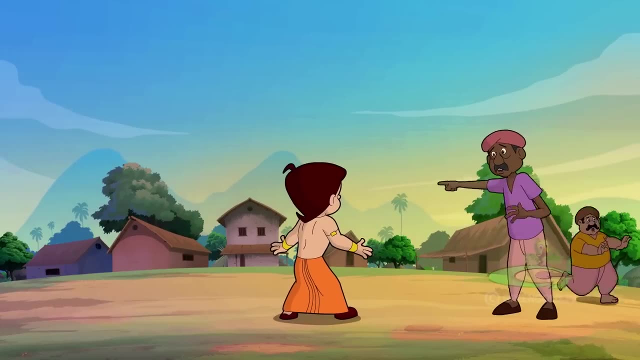 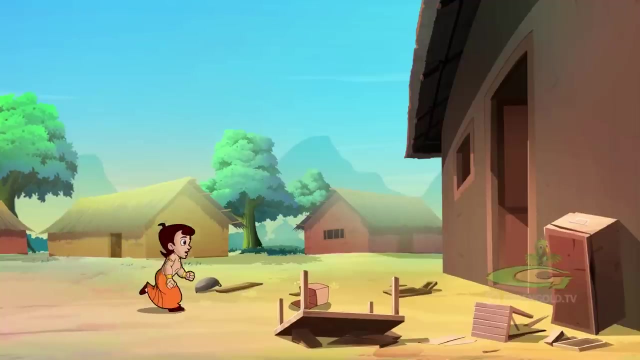 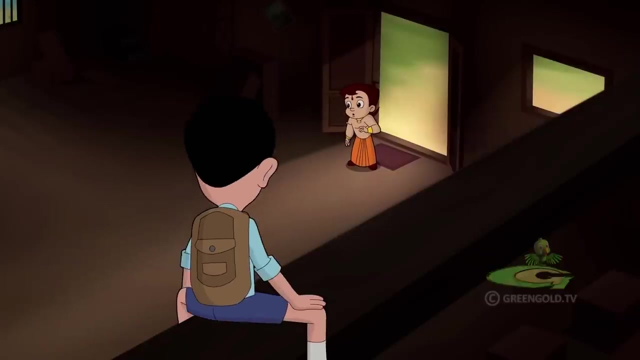 You need some pass for us. Please help us. Yay, Save us, Save us. We had experiments out there. Oh no, Please help us. Please help us. But who's doing these experiments? I am doing them. Look over here. 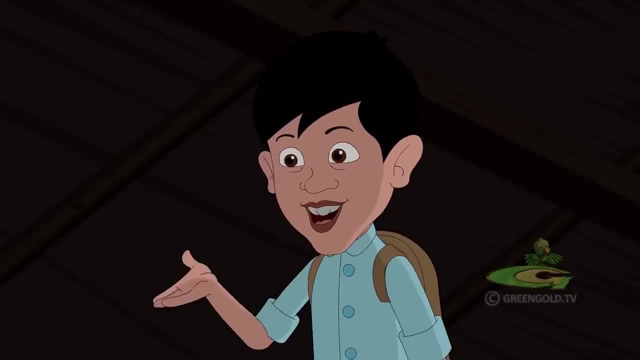 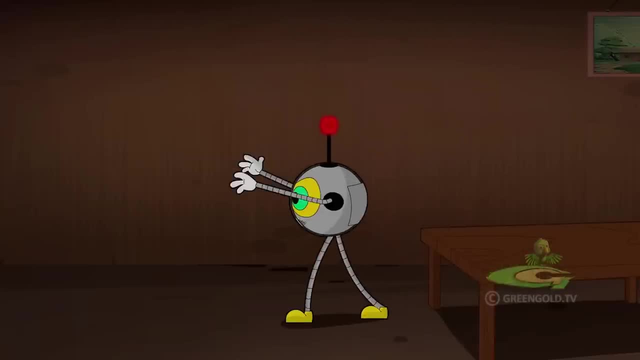 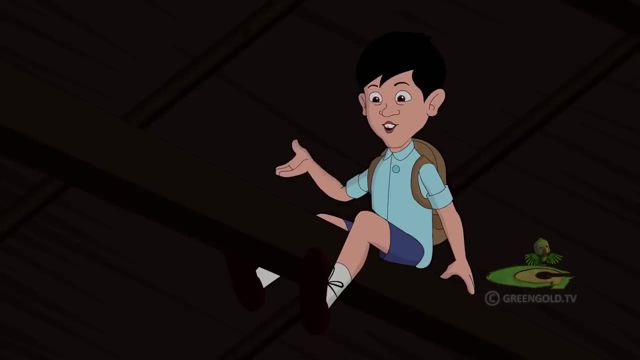 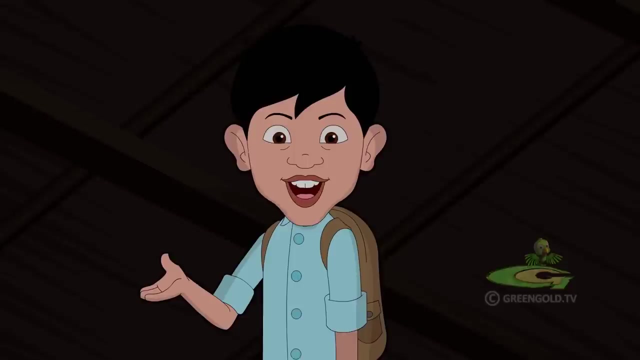 Clean up the house, Clean up the house. And this is my robot called Dumbo Dumbo. Why Dumbo? Because he's an expert in goofing up in every job he does: Clean up the house. Hey, Stop it. 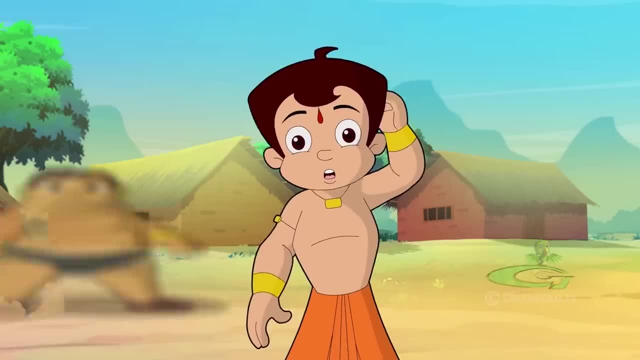 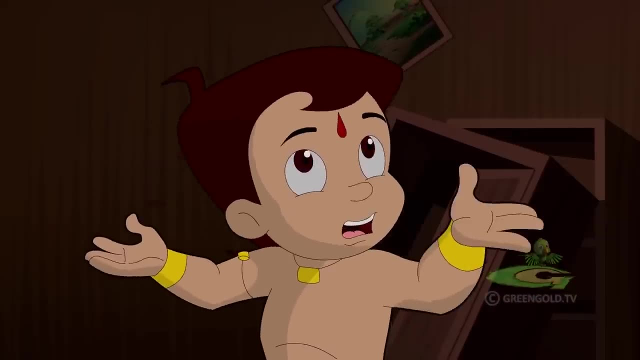 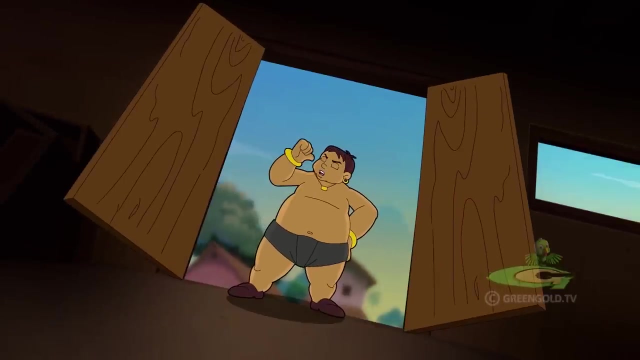 Clean up the house, Clean up, Clean up, Clean up. But why is he throwing out everything? Because I have given him the order to clean up the house, Clean up, Clean up, Clean up. Only Kalia can fix him up. 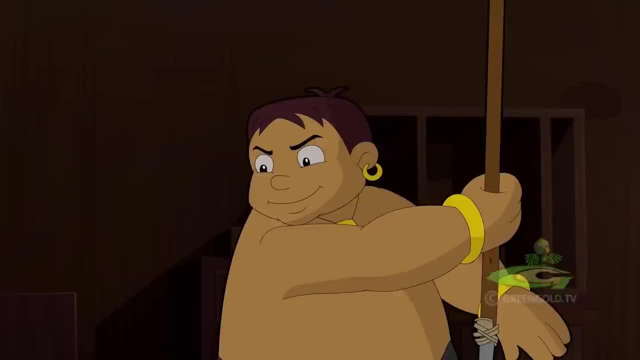 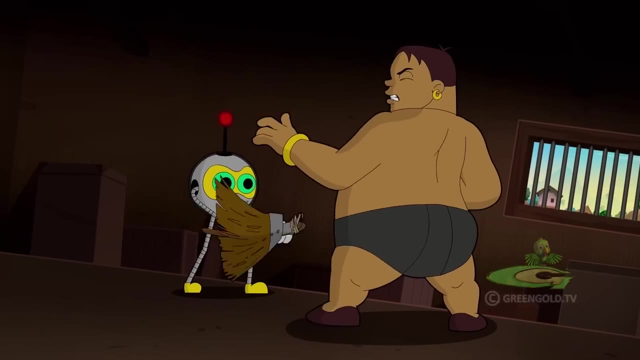 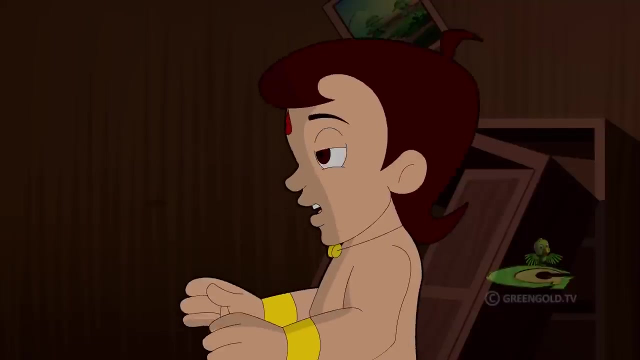 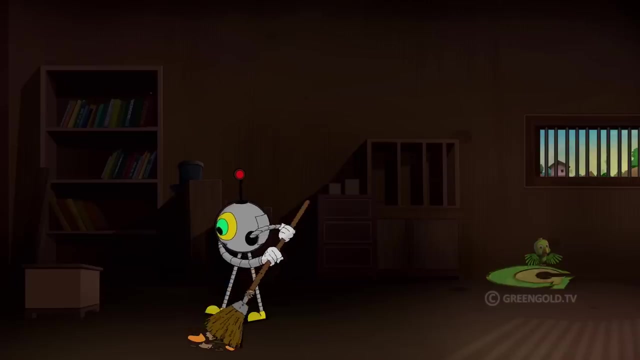 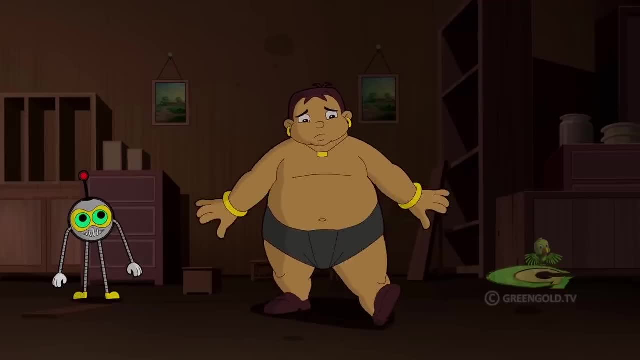 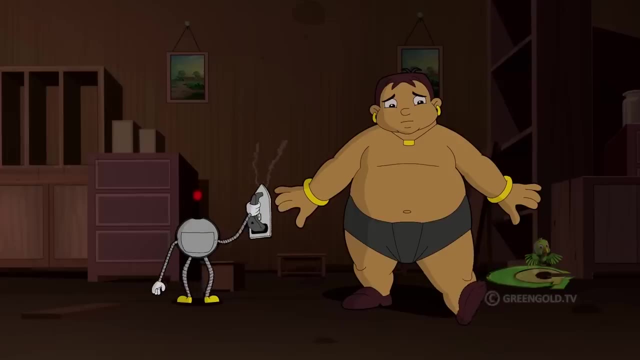 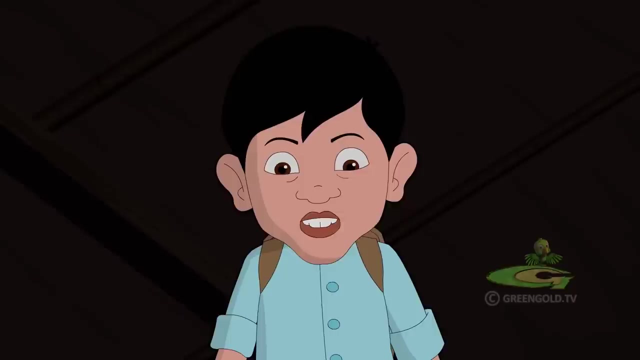 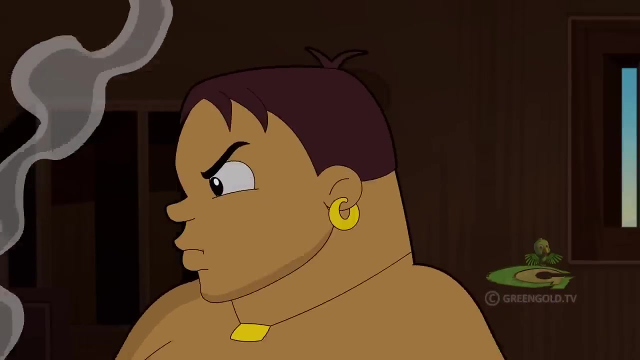 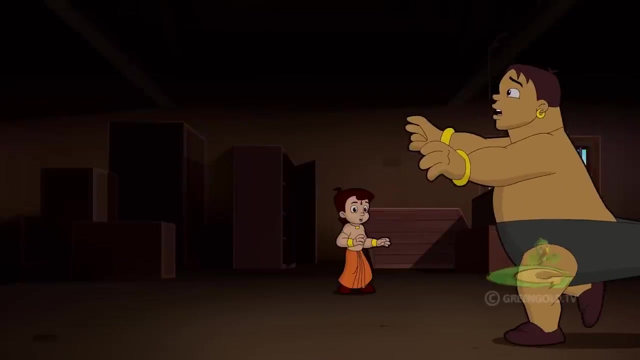 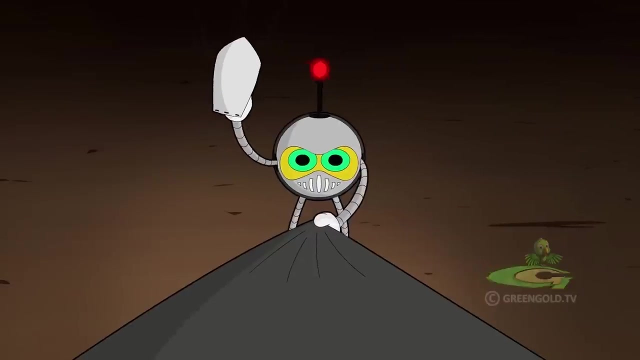 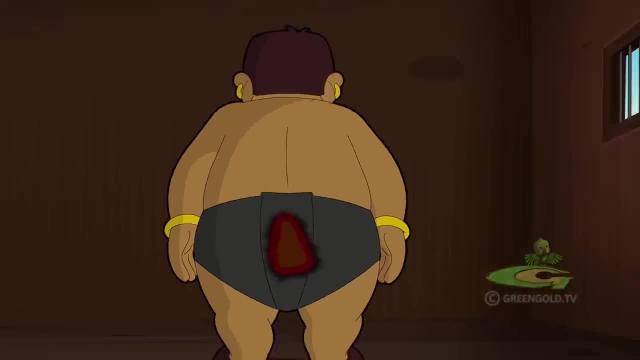 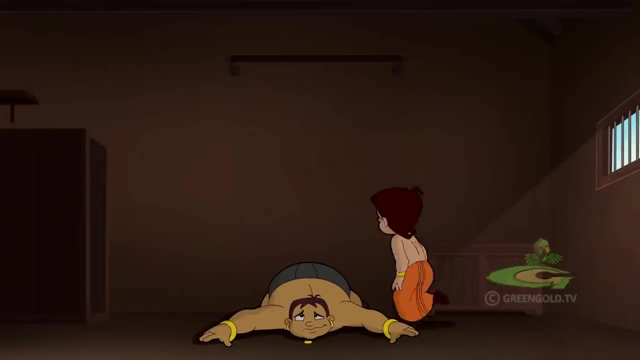 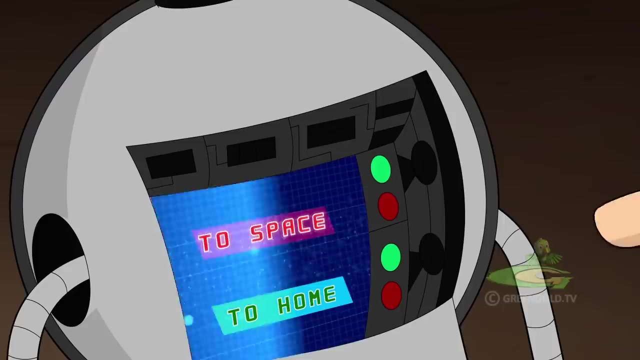 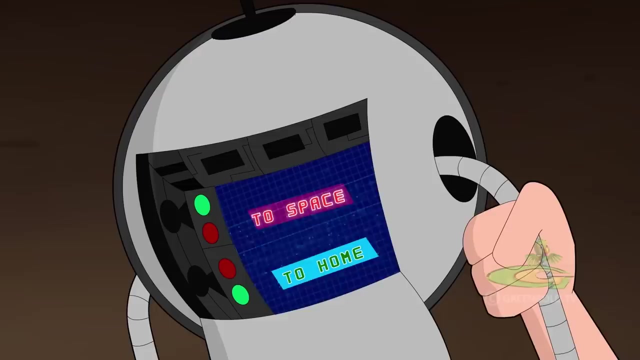 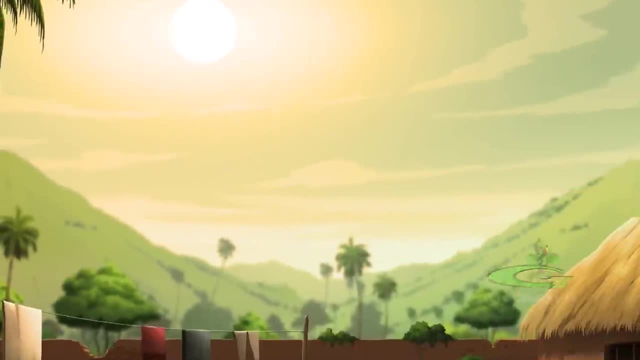 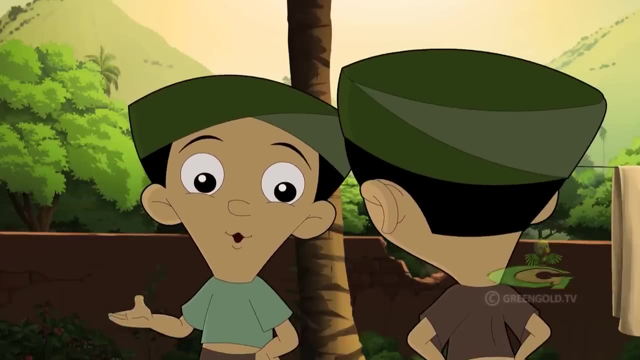 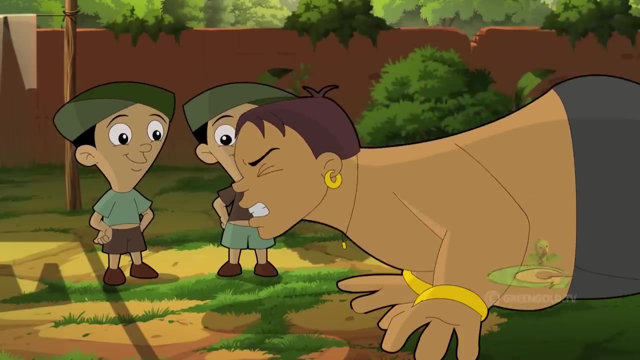 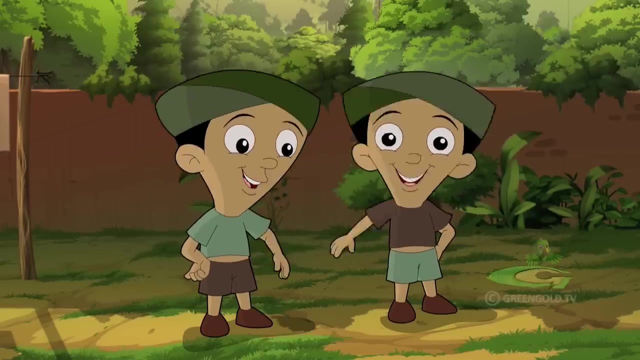 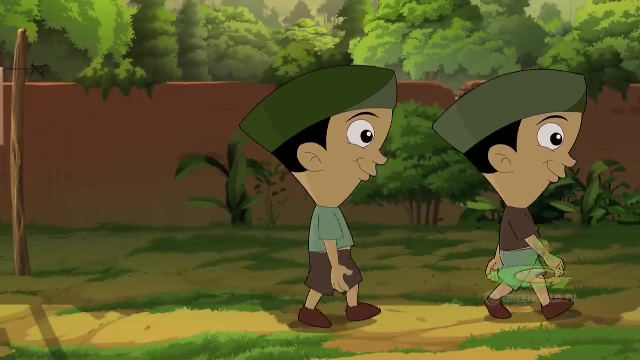 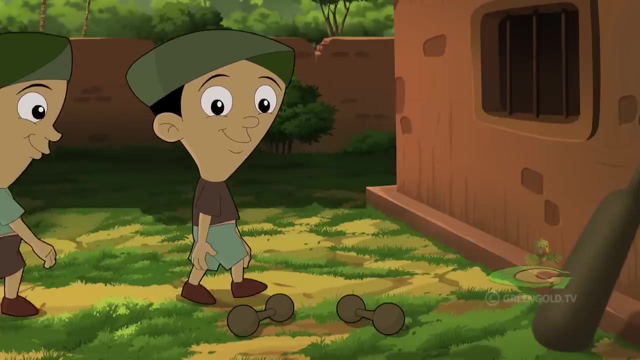 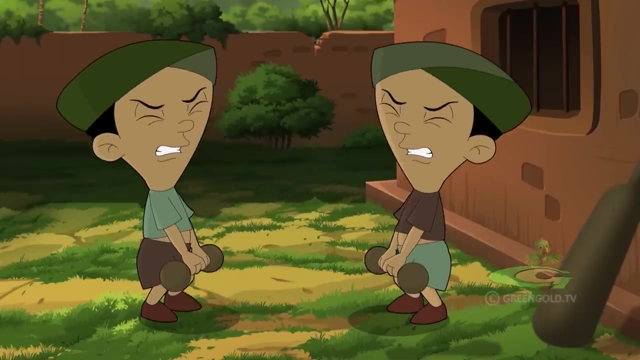 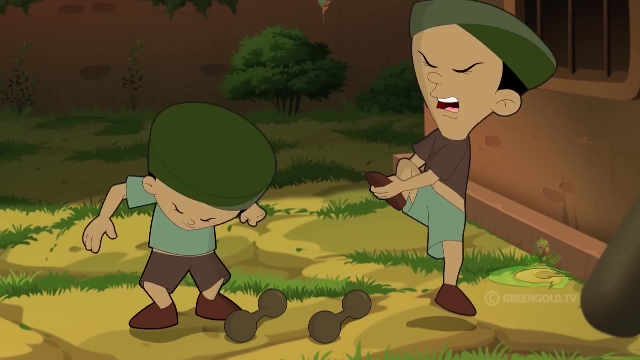 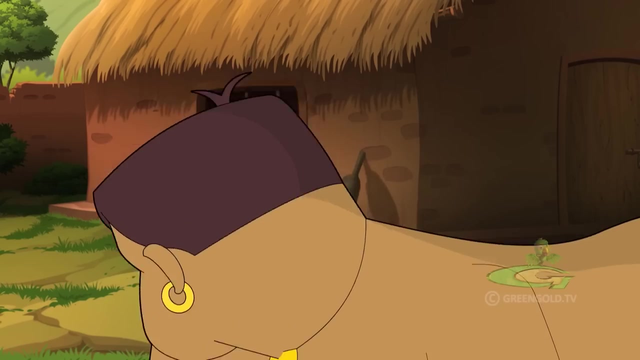 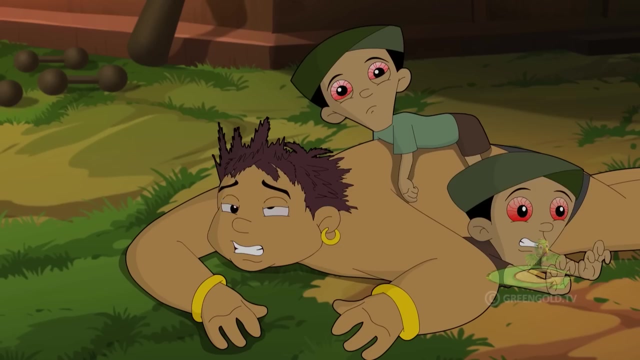 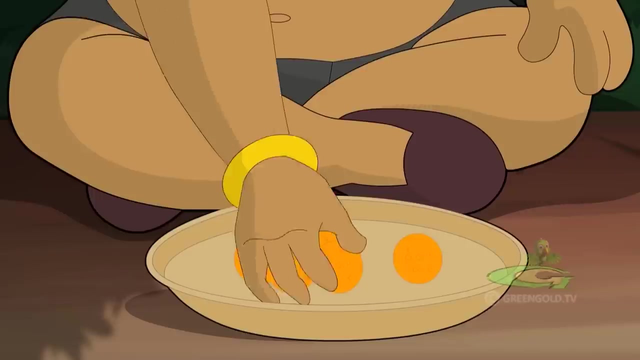 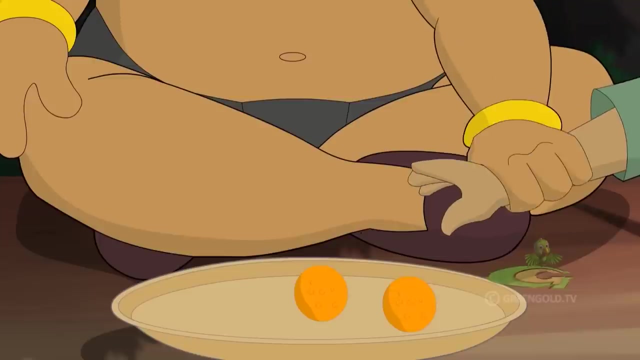 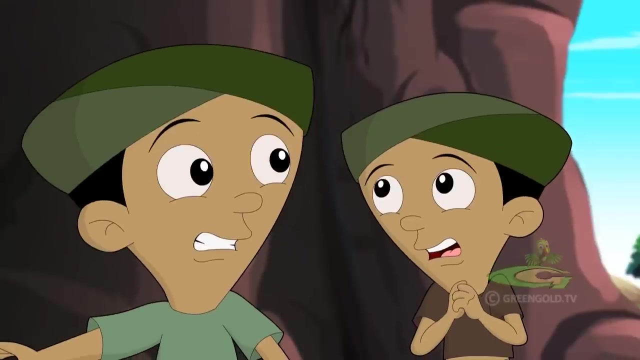 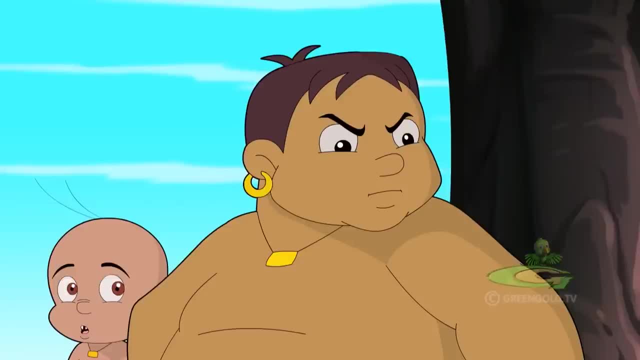 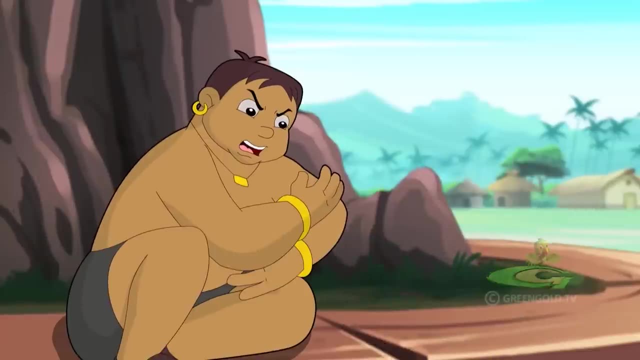 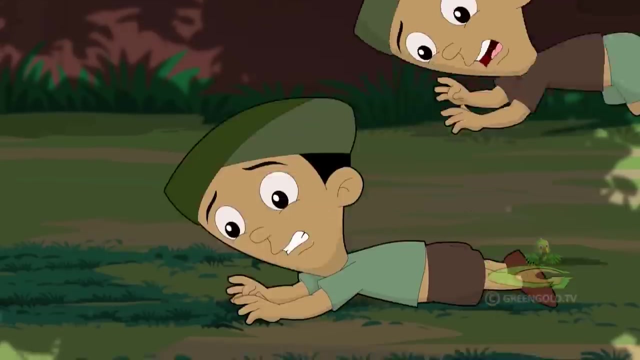 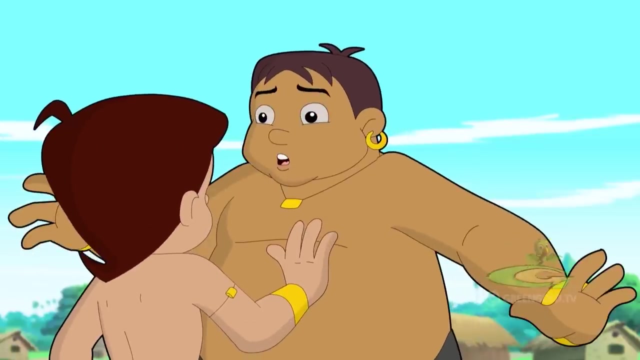 Though I don't know about the numbed, but you're definitely not just a skull. You both are going to have it from me. Stop, Stop, both of you. Come on, Kaalia, let them be. Why don't you do your work and let me and my boys do whatever we want to? huh. 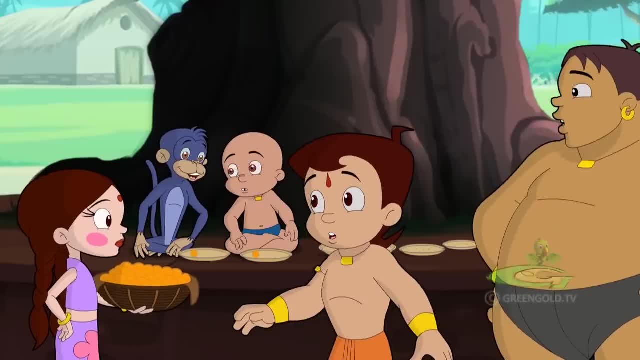 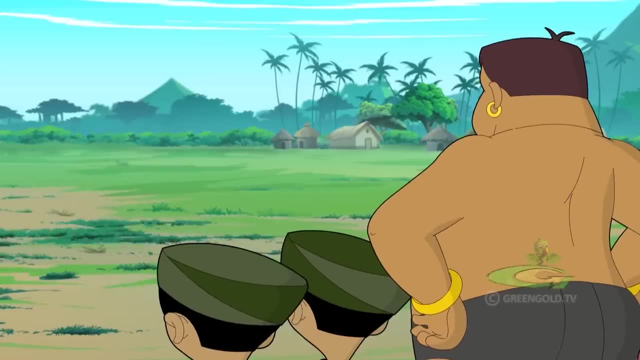 That reminds me, Bheem. Professor Dhoomketu had called you to his laboratory for some work. It's about something called a lava car. Everyone just calls Bheem all the time. Why doesn't Professor Dhoomketu ever call me for any work? 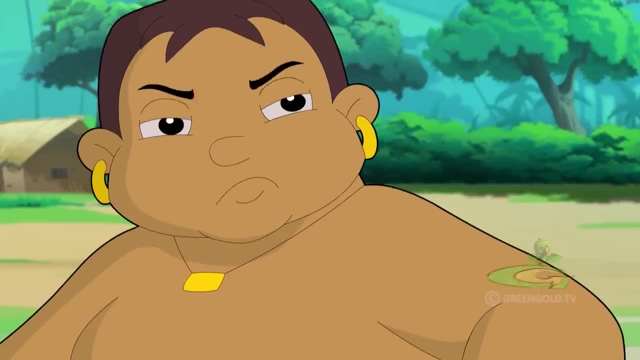 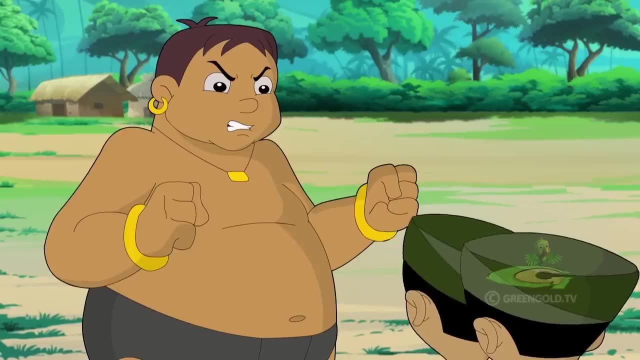 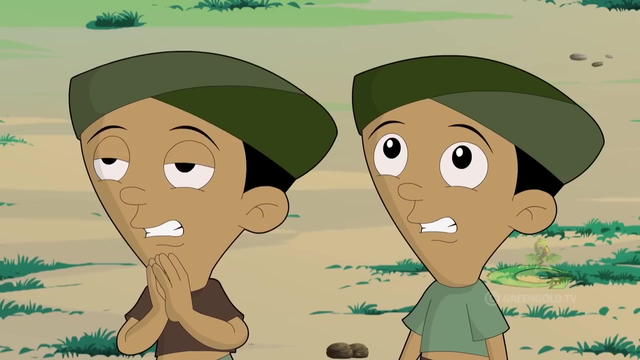 Had that been of any use, he would have surely called: What did you just say? I was just saying that you're the one and only world famous wrestler of Dholakpur, So you can walk in uninvited anywhere. Kaalia boss. 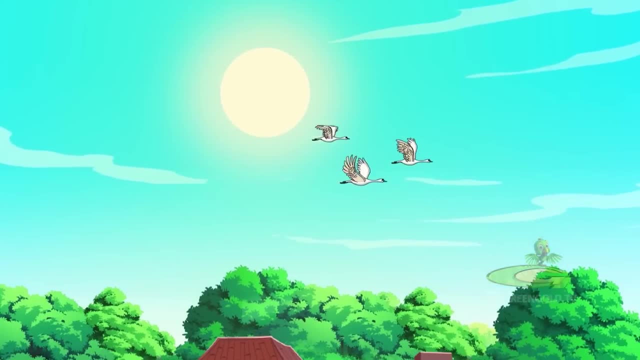 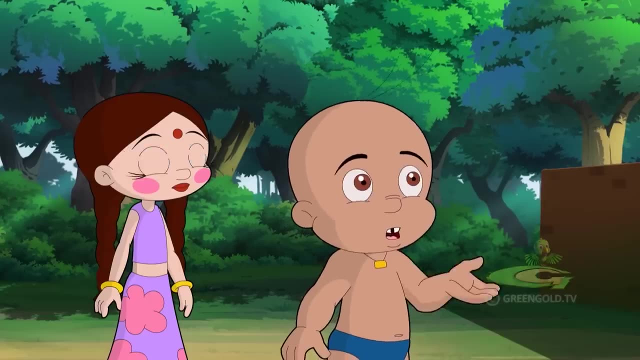 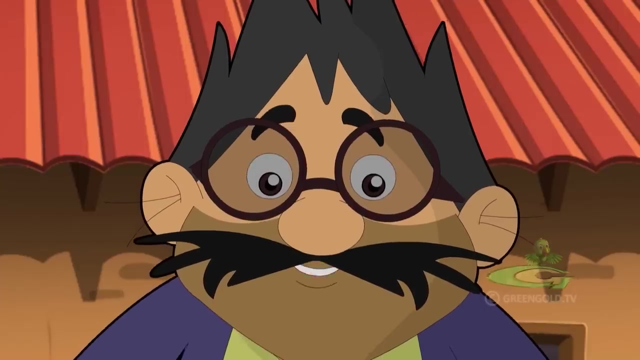 You got a point, So let's go. This is my lava car, But where is the lava uncle? Well, kids, if I had really put boiling lava into this, do you think making this machine- I mean this car- would have been possible? 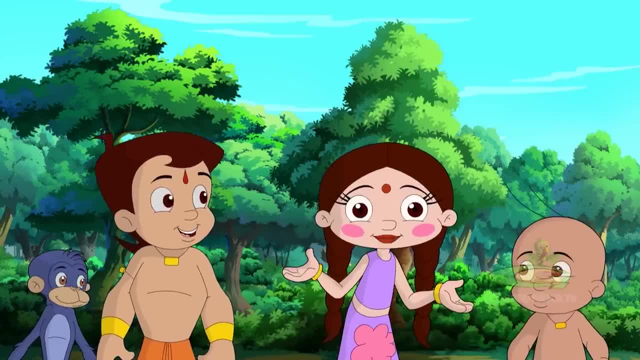 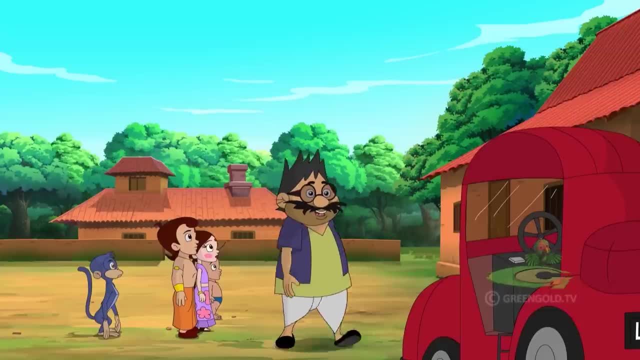 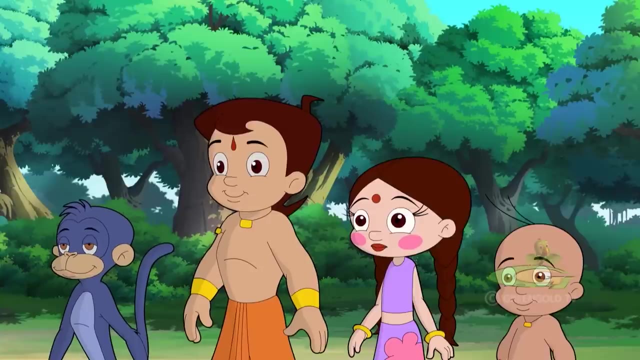 Of course not. Hot molten lava can even melt steel, And when it cools down, it becomes solid and heavy as a rock. That is why, instead of using actual lava in this car of mine, I have used certain new chemicals which mimic the properties of real molten lava. 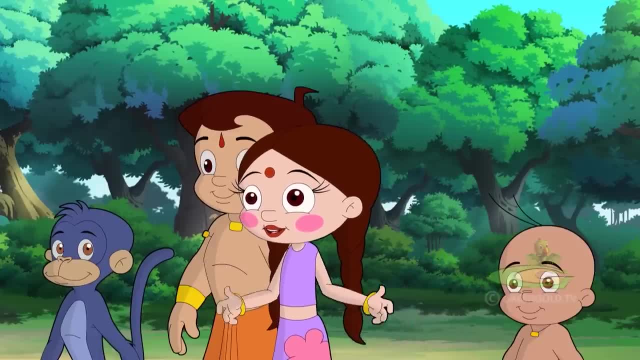 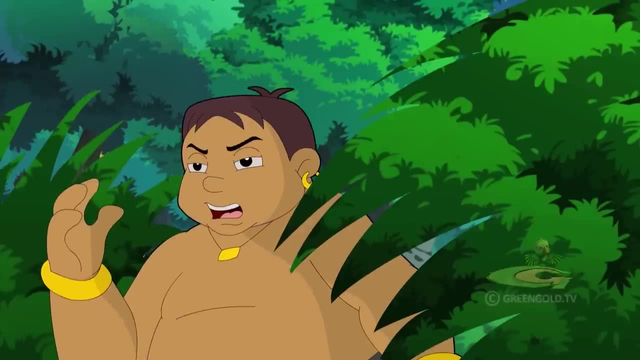 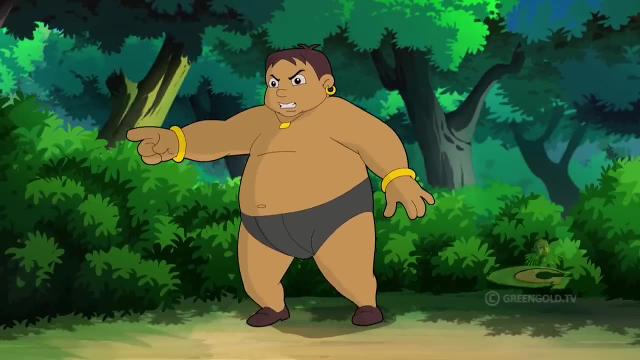 But what does this car actually do, uncle? Well, actually I have made this for cars, For car racing, you see, For car racing. Listen, I was thinking, if you can trial this car out, Bheem, Why Bheem, Why not me? 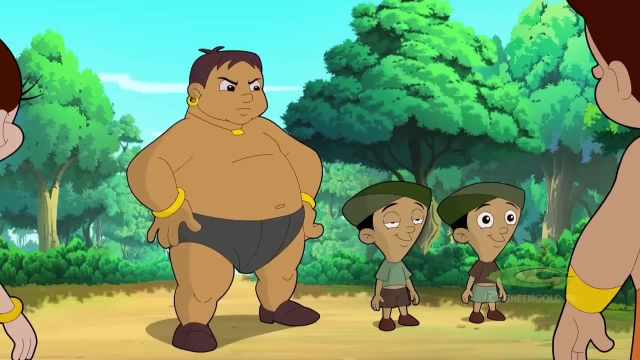 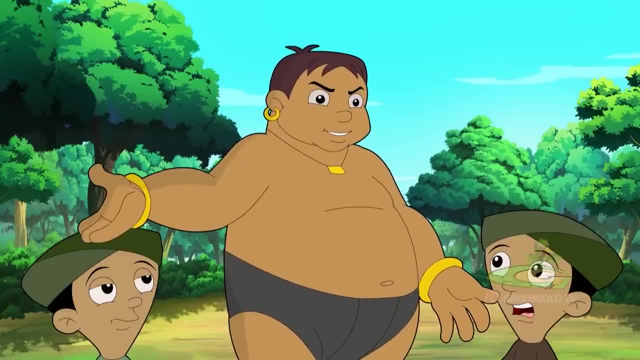 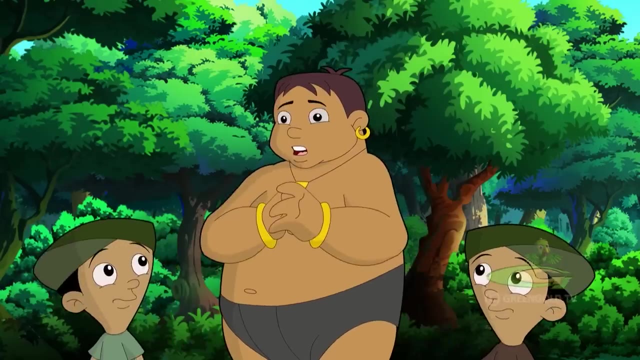 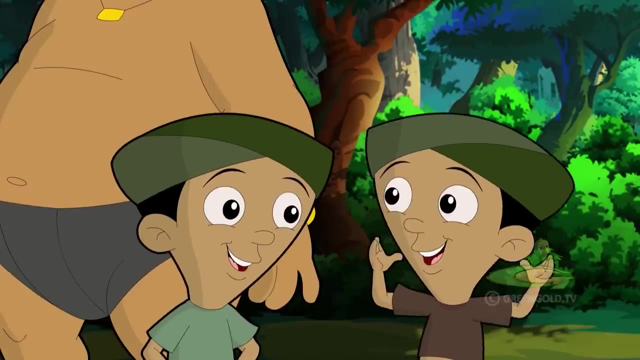 Kaalia. what were you doing behind the bushes? He was hiding and listening to what you were discussing. If anyone gets to trial this car first, that should be me. He would be able to understand the intricacies of this car Instead of understanding intricacies. boss understands delicacies better. 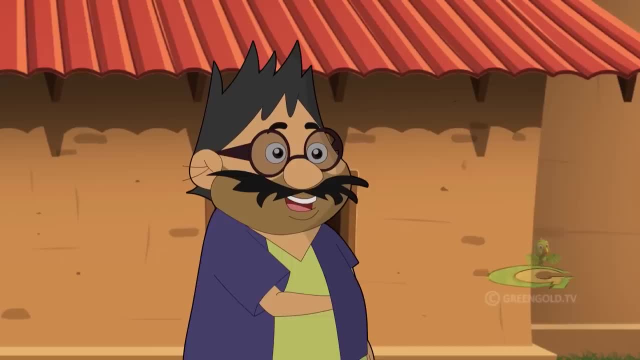 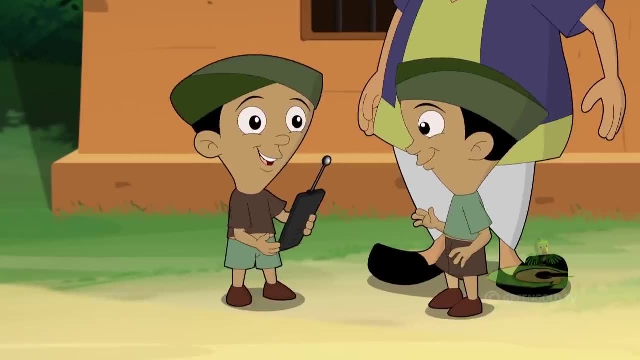 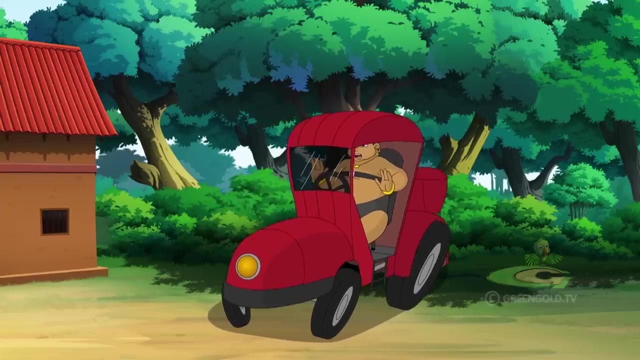 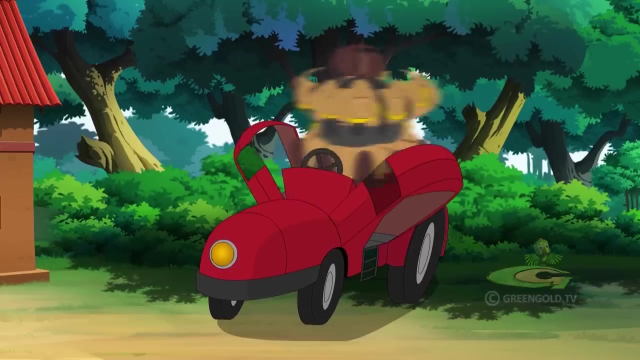 Although all the controls are inside the car, but for the sake of convenience, I have made this remote for it, Which would be used by us. Come down, Dholu Bholu, Enough now. Dholu Bholu, stop it now. 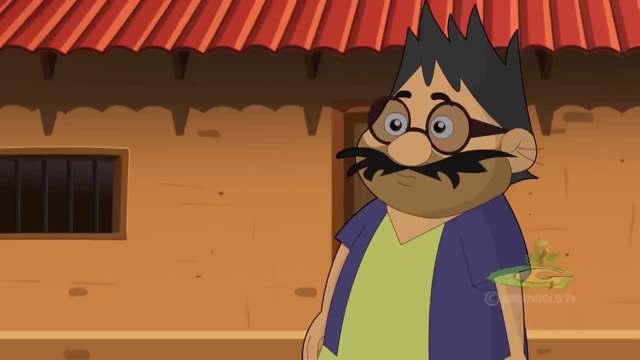 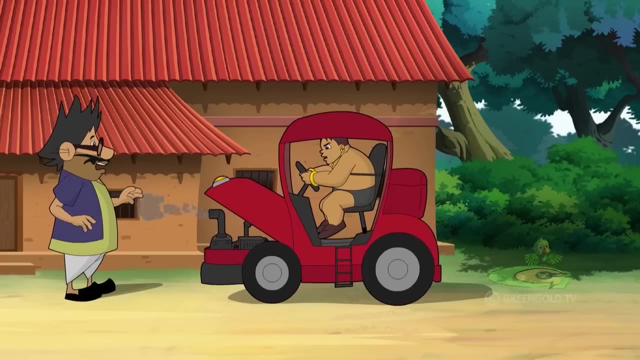 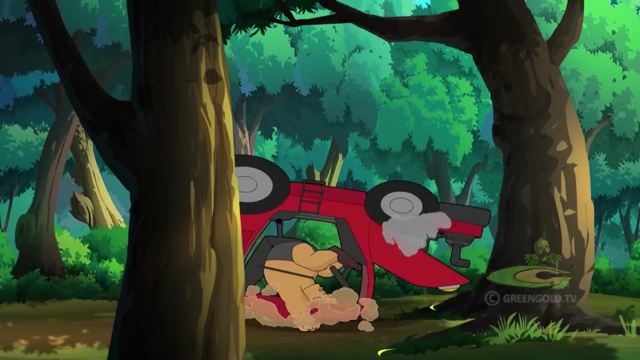 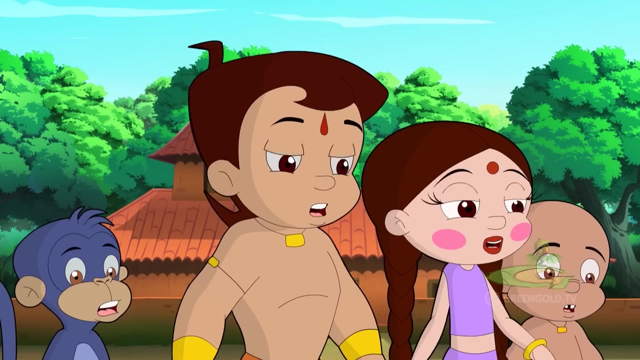 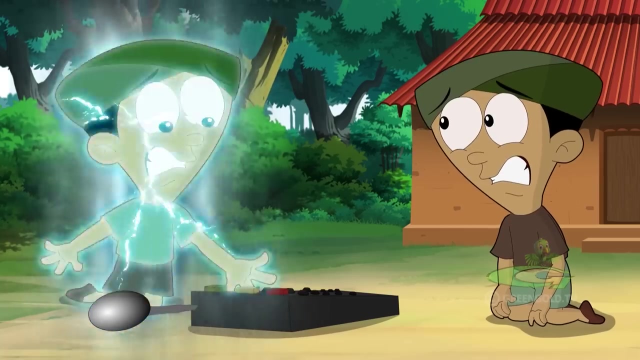 Come on, why can't we both have a little fun? Bheem, We are just trialing out everything in this new car. Mom Kaalia, Mom, Crazy smoke, Oh no. What's this Yikes? Oh no. 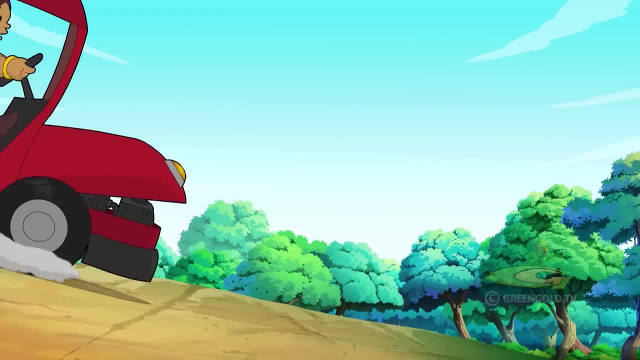 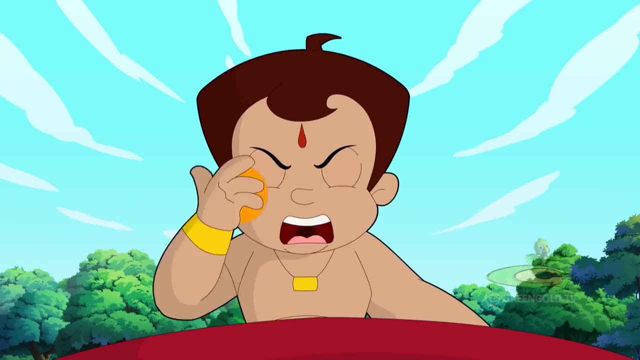 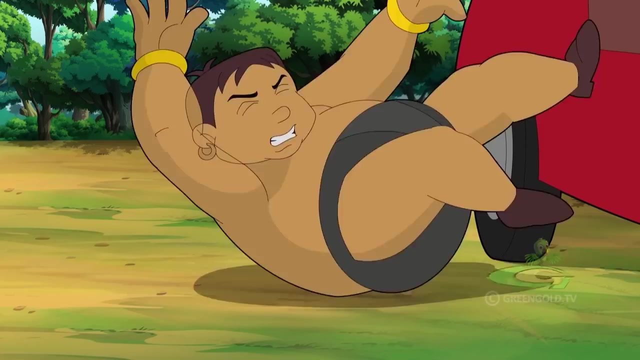 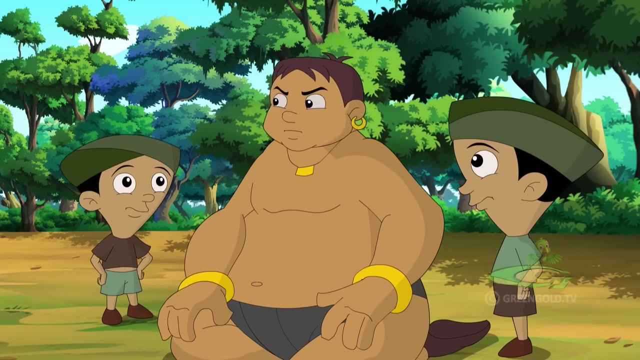 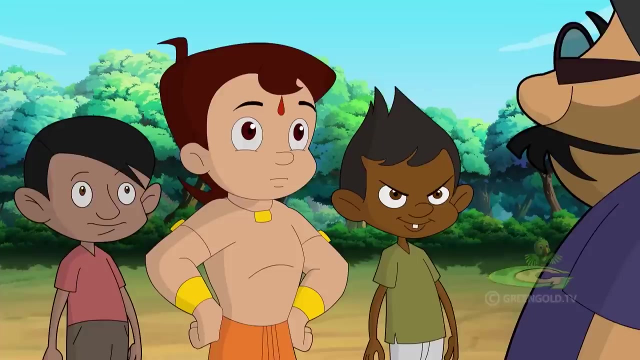 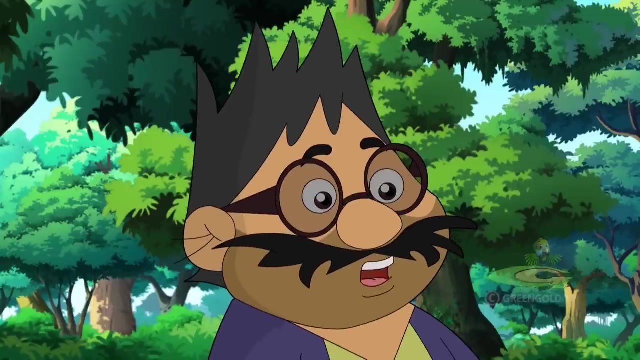 Move out of the way, Bheem, Take this, Don't worry, Everything is fine. Bheem, hope you didn't get hurt. And how's Kaalia? Yes, we are fine, But your car? Well, let me take this vehicle back to my laboratory. 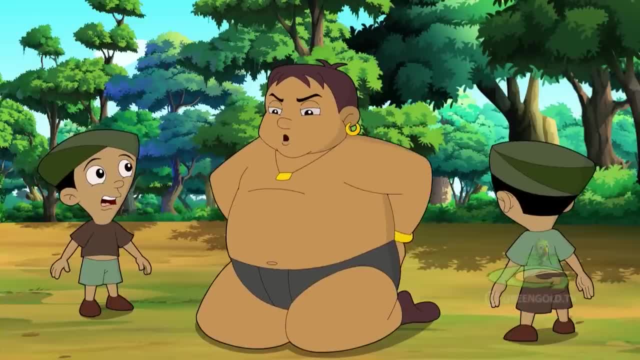 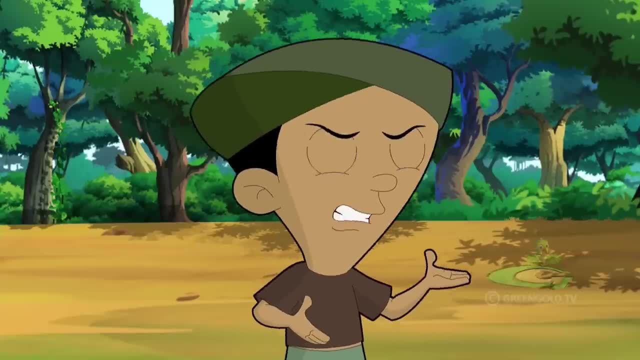 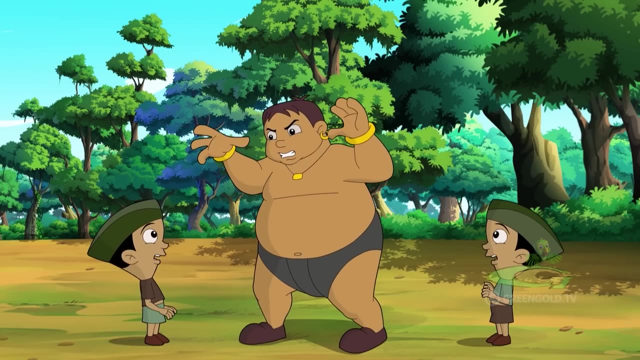 Oh, my bones are aching so badly. Do you really have any bones? I thought it's only fat in there. Okay, Okay, You can take it, You don't need to worry. No, Claire, Yes, Well, I see. 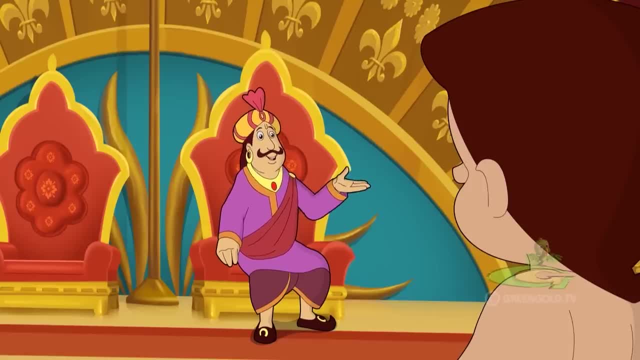 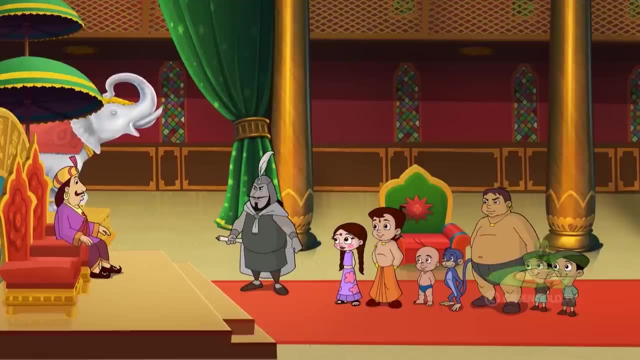 Well, I see You're going to get some rest. alright, Sure, You won't be able to stay for long. Yeah, sure, Ma'am, I'm ready to go out. I'll see you later. Okay, see you later. 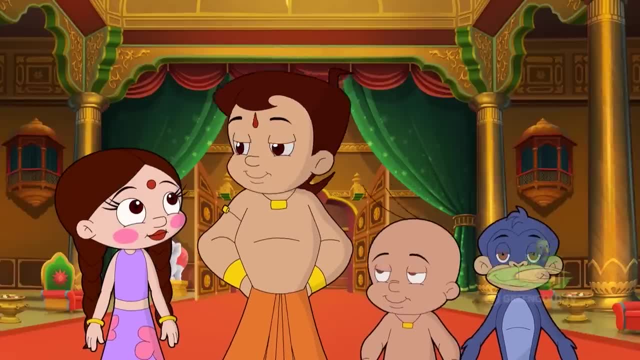 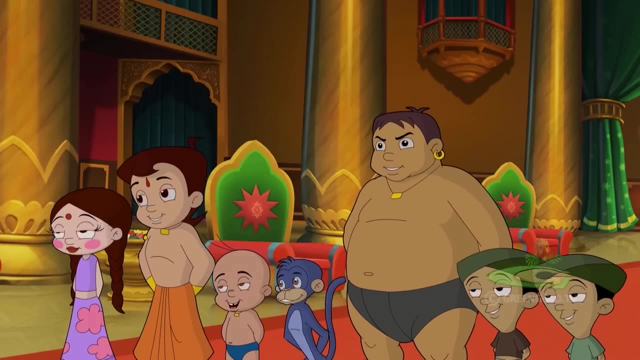 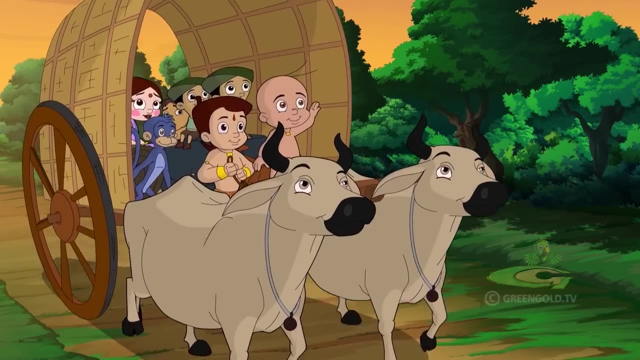 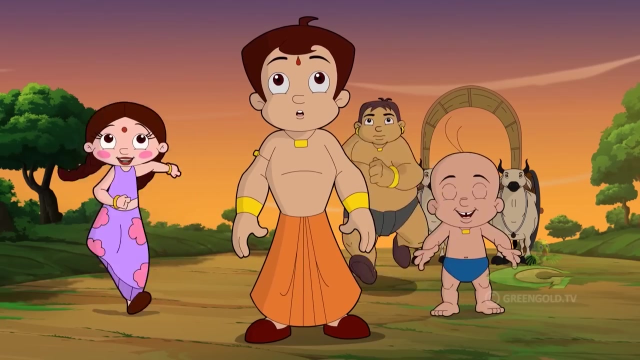 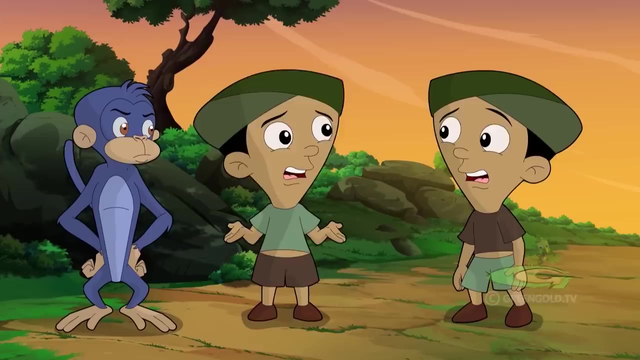 Okay, Bye, son, small gift from me. I am sure you are all going to enjoy this camping trip. So are you all willing? Yes, my lord Neeli Pahadi. Wow, This is nowhere close to the color blue. 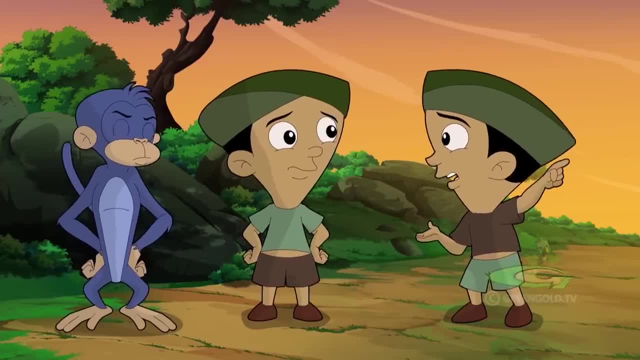 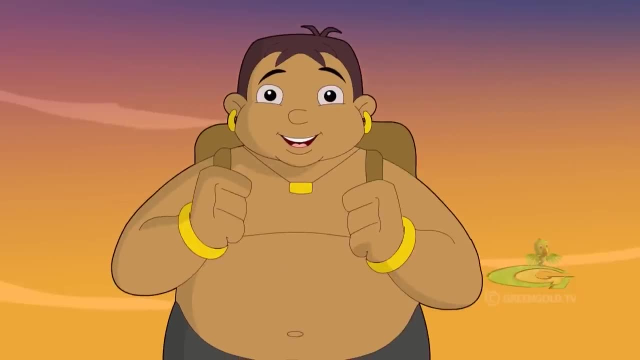 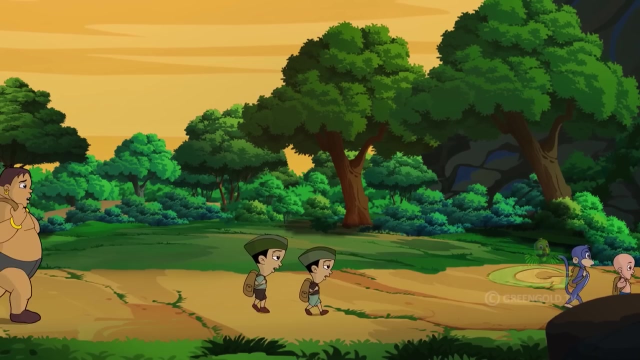 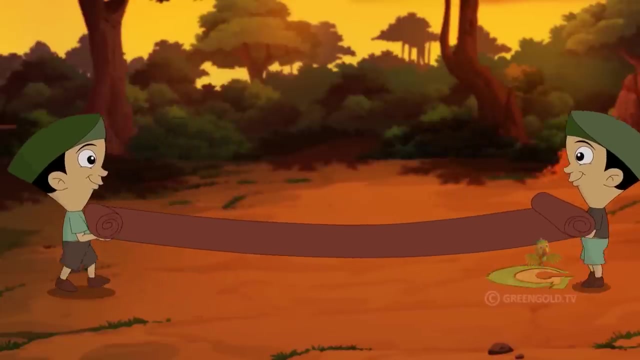 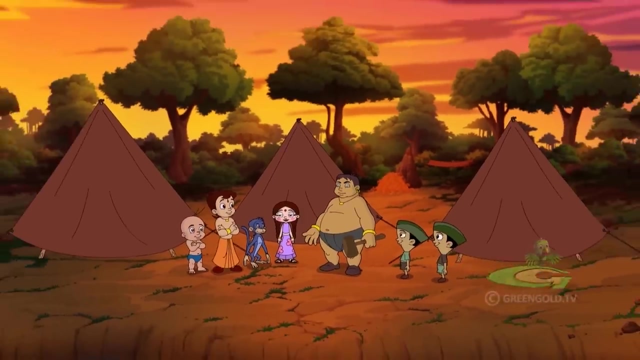 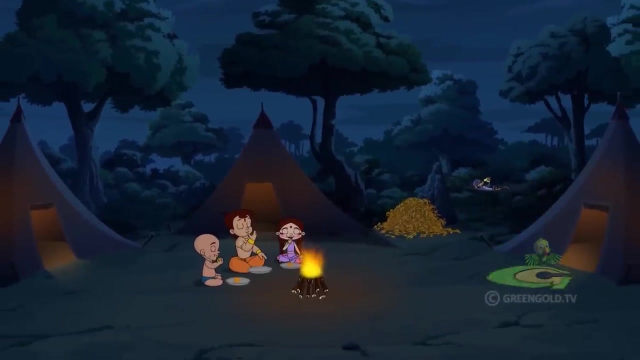 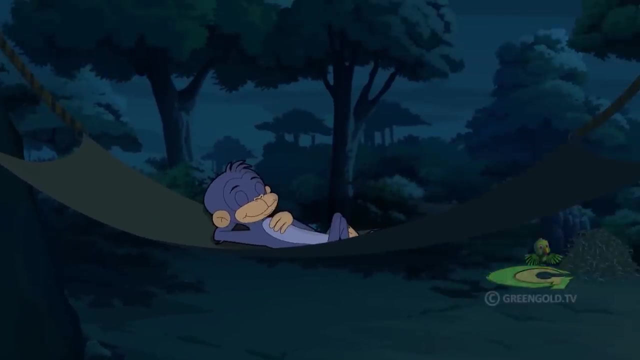 Then why is this called Blue Mountain or Neeli Pahadi? You fools, That's just a name, A name. The other side is Razoru Mountain. You vs Neeli Pahadi, I don't know. ். Having ladoos at night is much more fun, guys. 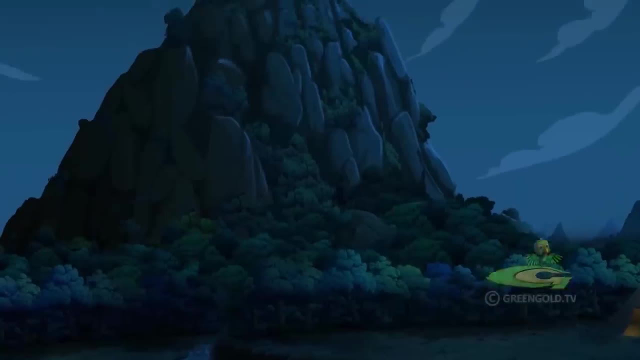 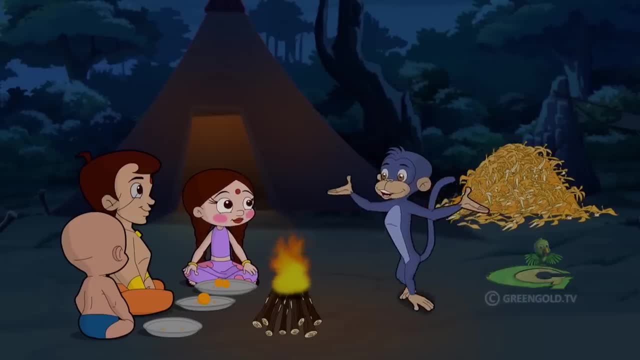 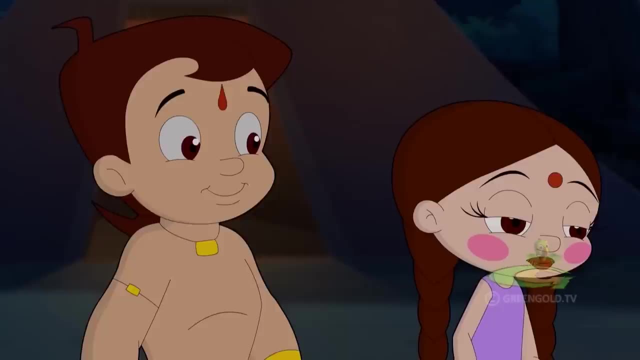 From the next one we are going to-. We are here to have fun, not to climb on top of a mountain. It's quite late at night. I'm feeling very sleepy. I'll be on guard duty. all of you go to sleep. 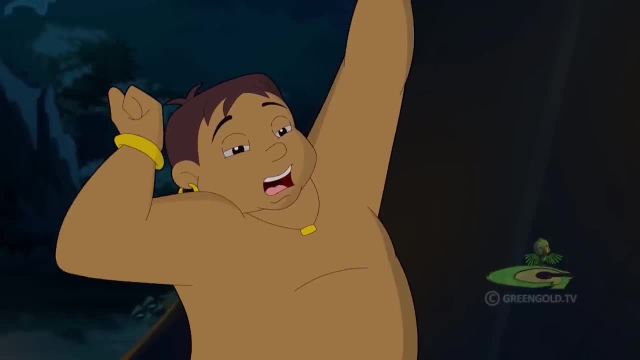 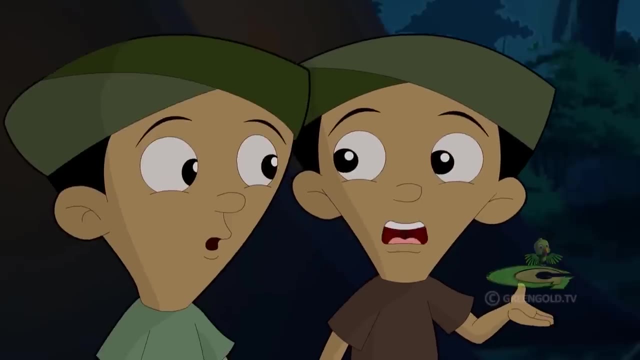 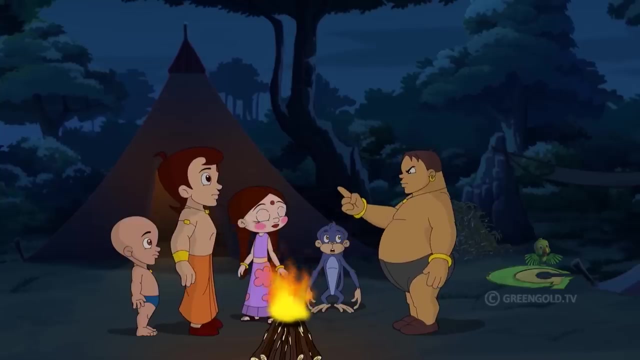 Let's go to sleep, then. Bheem is protecting everyone, even here, Like he does at Dholakpur. Let me do the guarding, But Kalia Bheem Neelipahadi's expert is Kalia the wrestler. 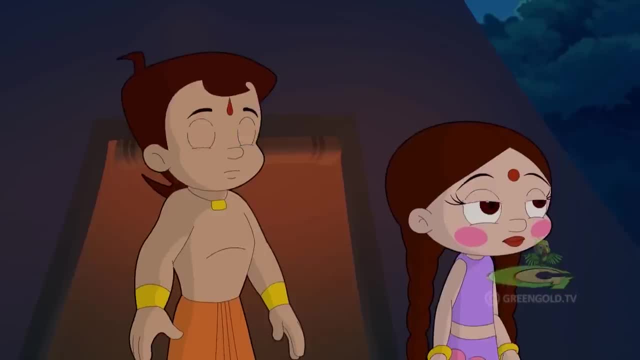 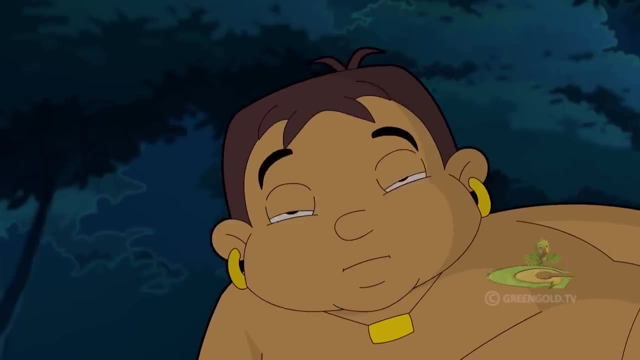 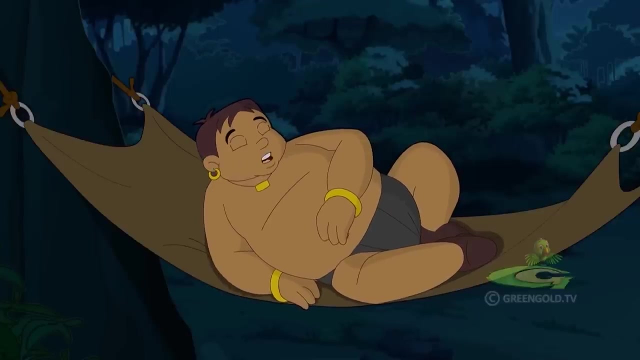 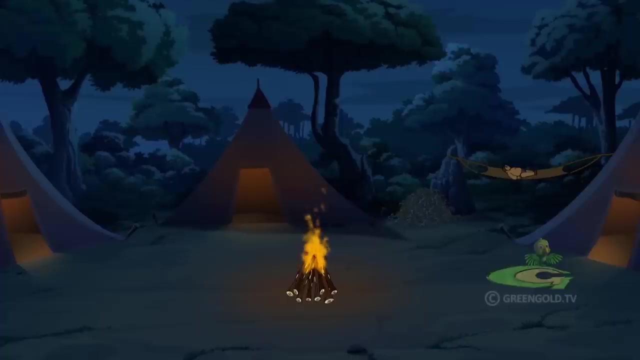 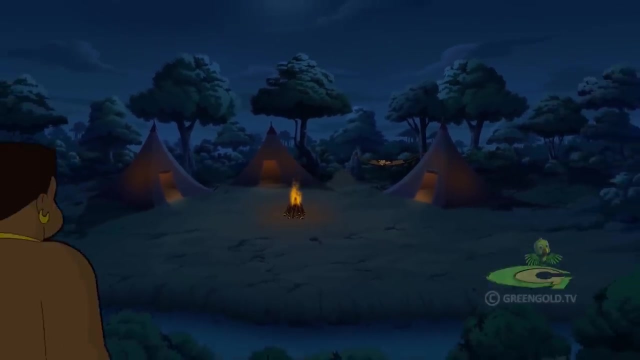 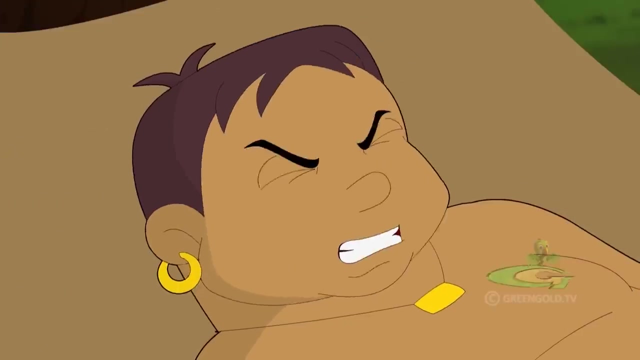 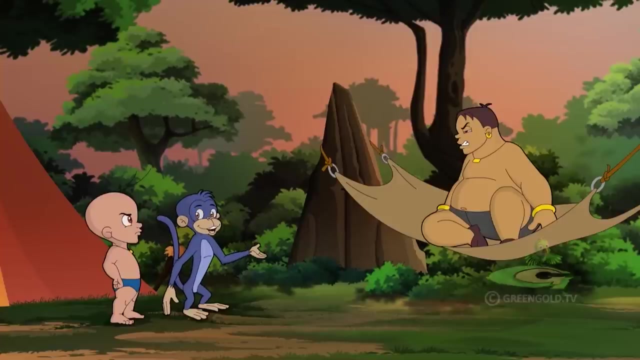 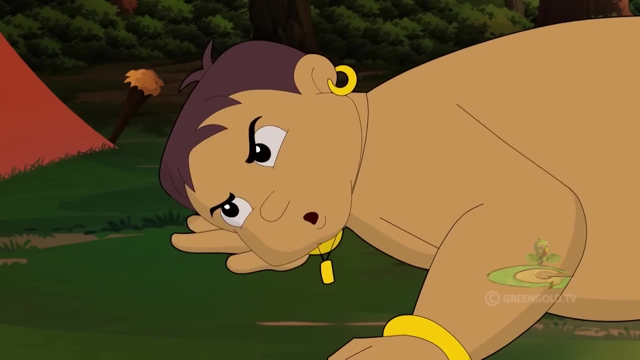 I'll do the guard duty. rest will sleep. I won't sleep Neelipahadi's expert. I won't sleep. Kalia, I'll do the guard duty And he's snoring away. What happened, Kalia? we have been robbed. 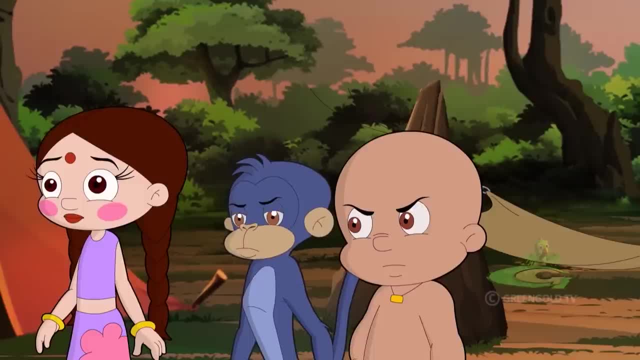 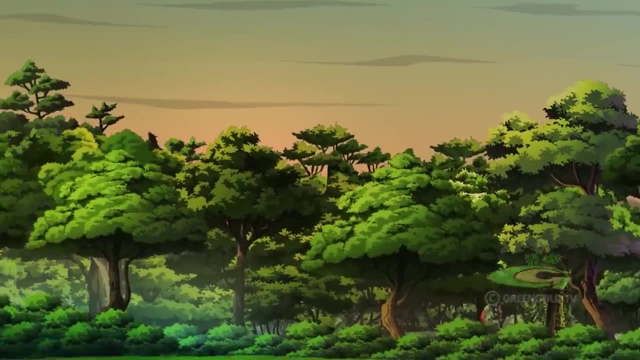 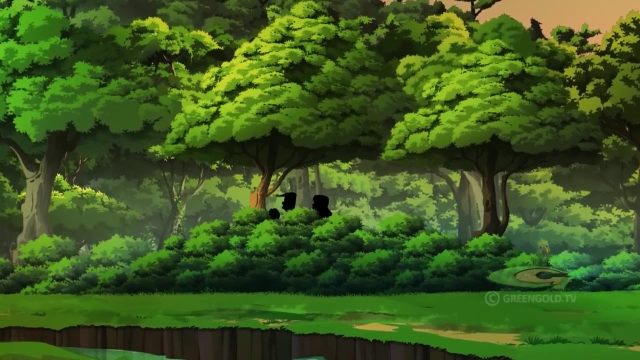 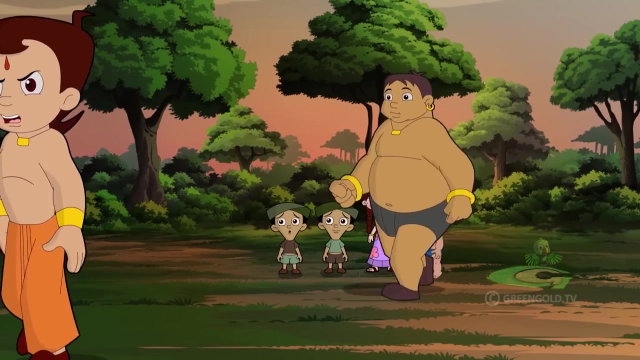 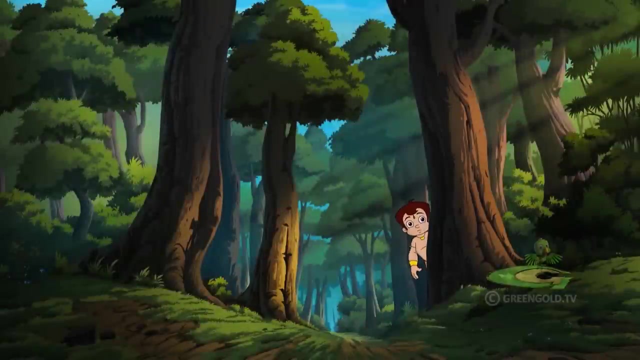 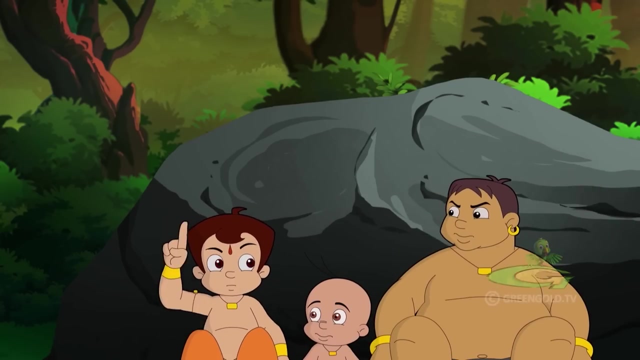 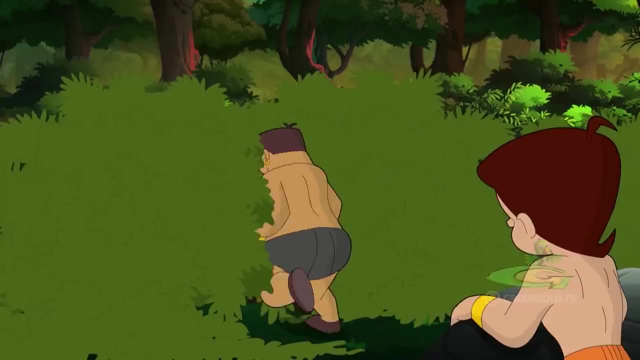 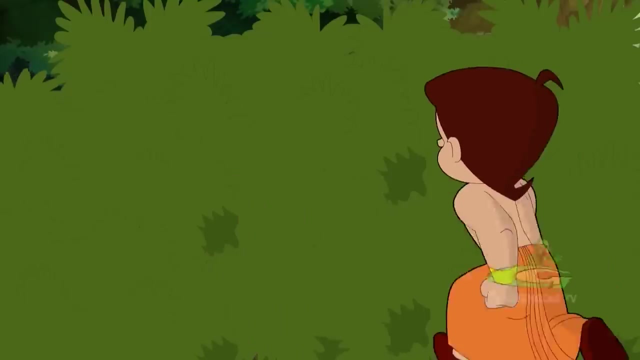 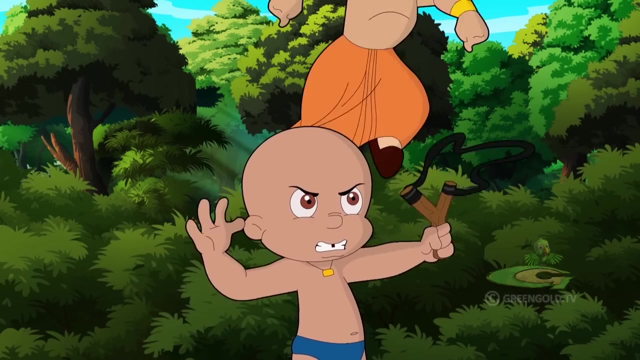 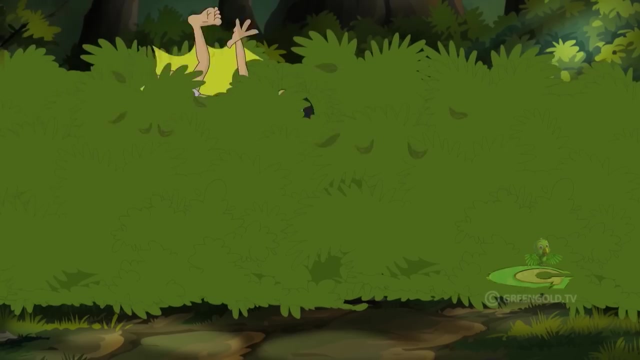 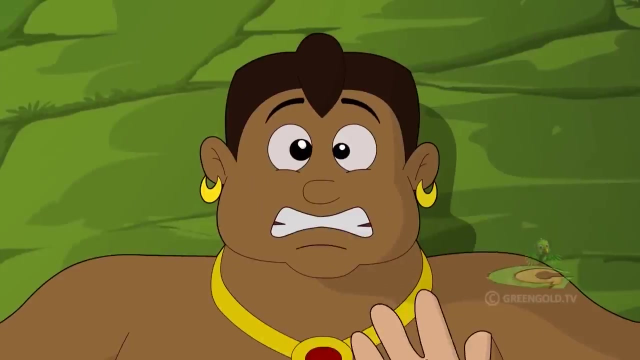 What? Someone else is also here. Bheem over there. Come on guys. Shhh, Catch the thieves. Pah Huh. Oh Keechuk, You guys and her Bheem, look all our camping stuff. 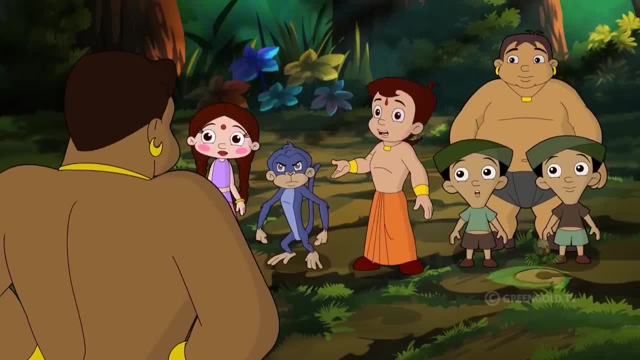 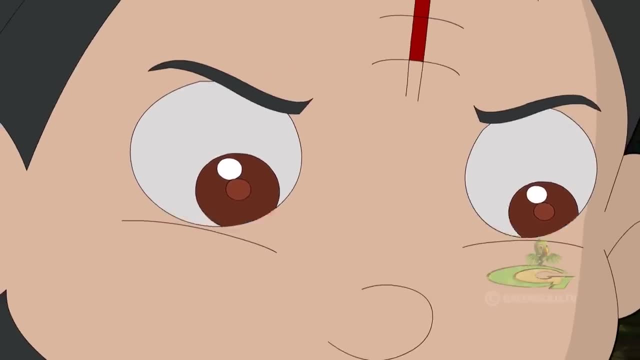 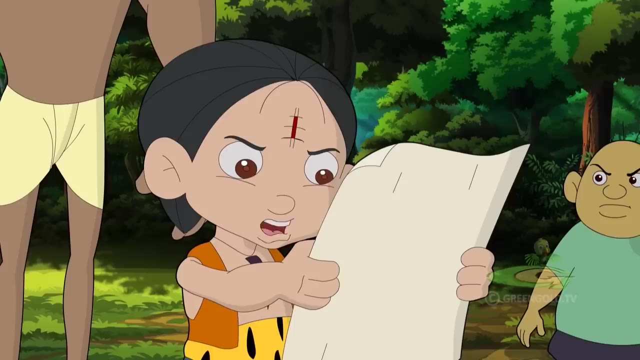 Huh, What are you doing at Neeli Pahadi now? Huh, What is this? Dholakpur's Bheem will scale Neeli Pahadi soon. Others are all buffoons By sending such a message to Neeli Pahadi. 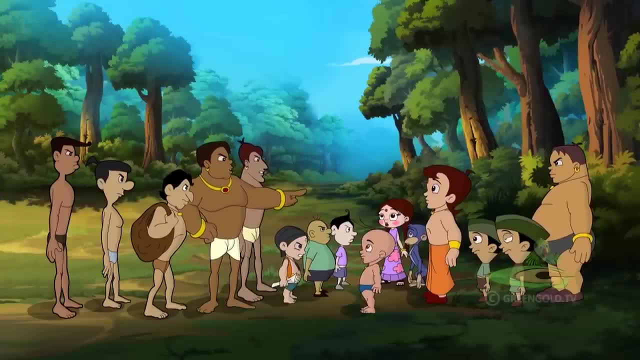 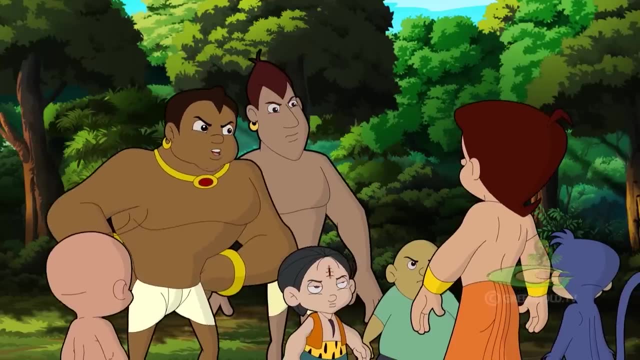 I'll get rid of her. By sending such a message to Pahelwaanpur, you've definitely insulted us. Bheem Keechuk, I'll never stoop so low. Now you're lying, since you're scared, Bheem. 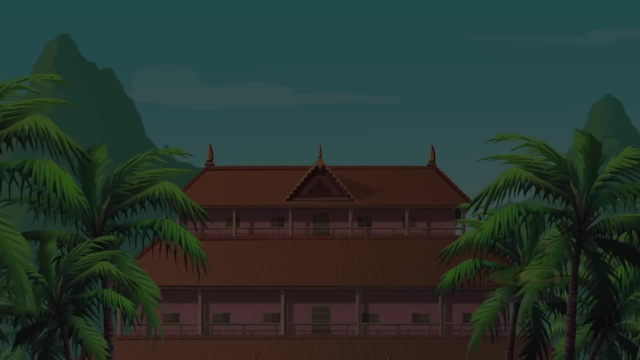 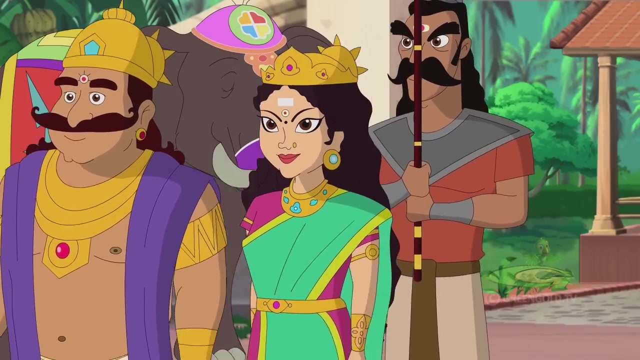 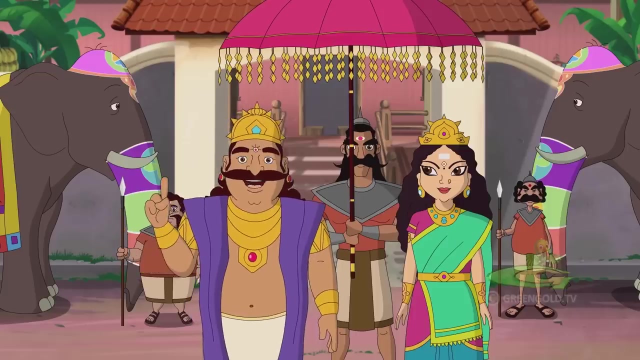 We've come here for a few days on a trip. Keechuk, My dear citizens of Kerala, today is one of the happiest days in all our lives. Today is one of the happiest days in all our lives. This ancient idol, which was stolen from our state. 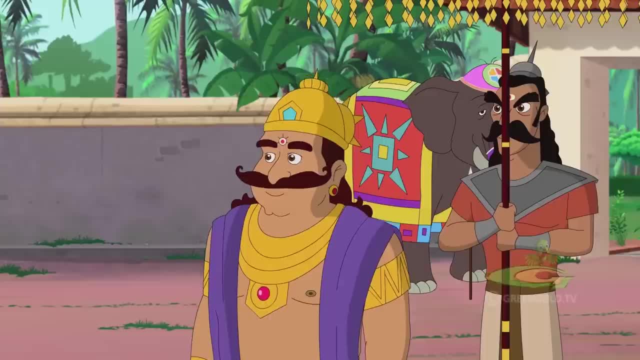 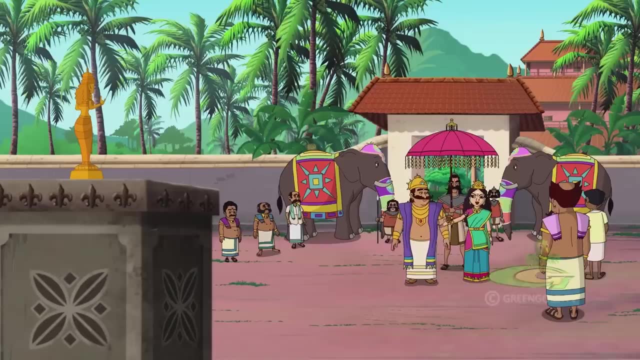 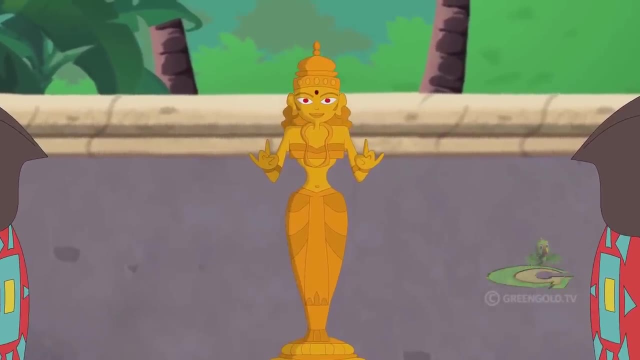 nearly a thousand of years ago- nearly a thousand of years ago- has been successfully recovered and brought back to our state after years of searching. This unique idol was the pride of our state and will always remain so and will always remain so. We will install it back in its temple. 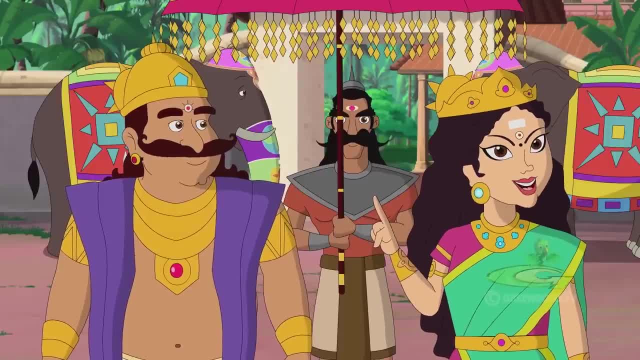 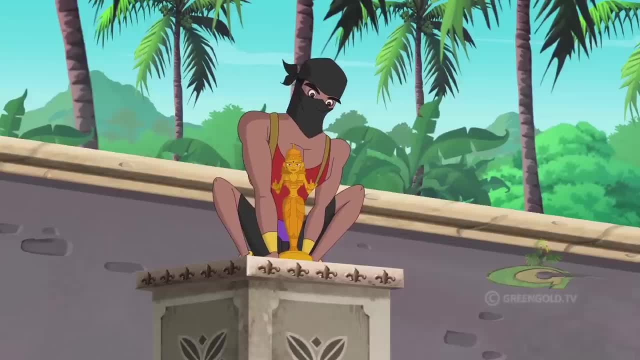 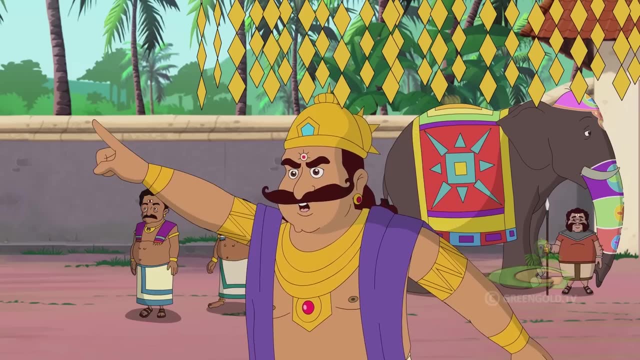 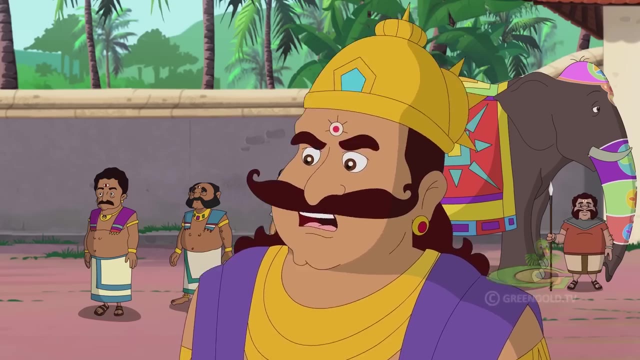 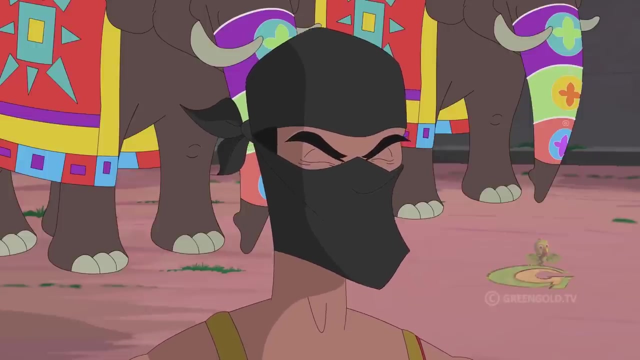 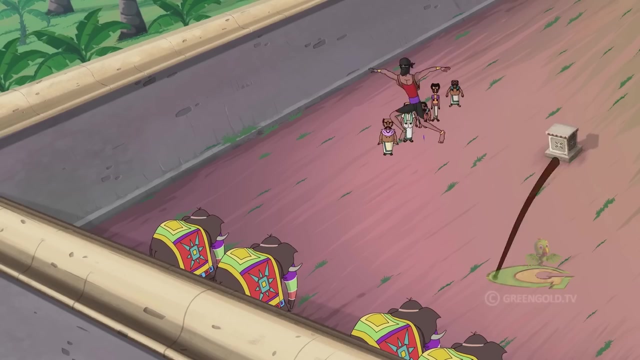 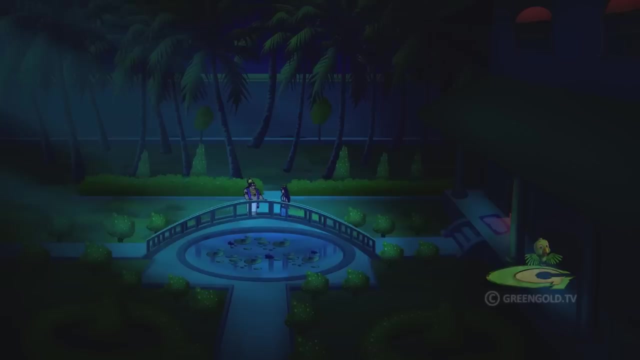 Yes, No one except me. Yes, No one except me. Yes, No one except me. Guards go, Guards go, Guards go. My lord, whatever happened is indeed very sad, but please don't waste, your time worrying. 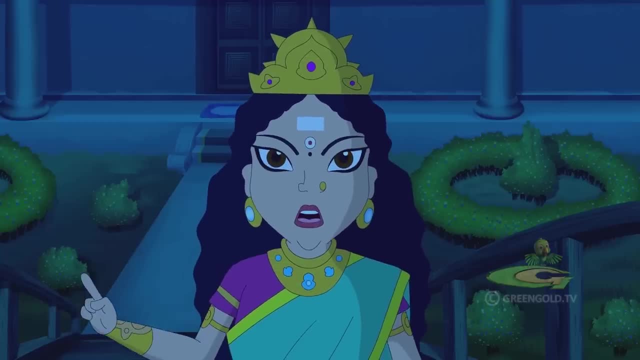 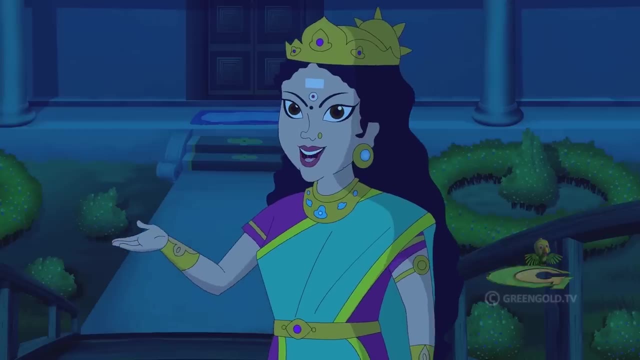 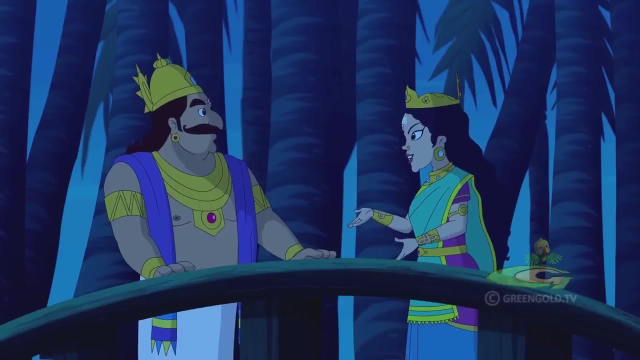 about it That unknown thief will be caught very shortly. All our people are waiting eagerly for the festival. Many more arrangements are yet to be made And this year the special invitation of the festival has already been sent to your friend, His Majesty of Dholakpur, King Indravarma. 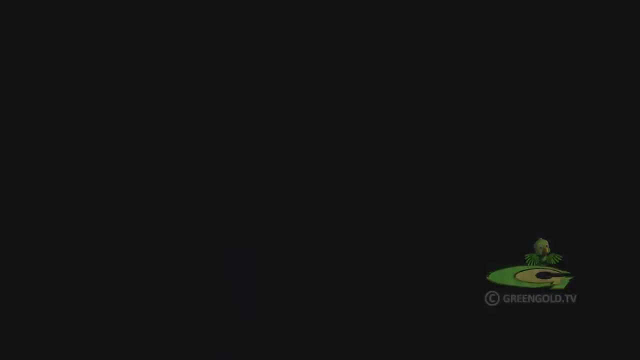 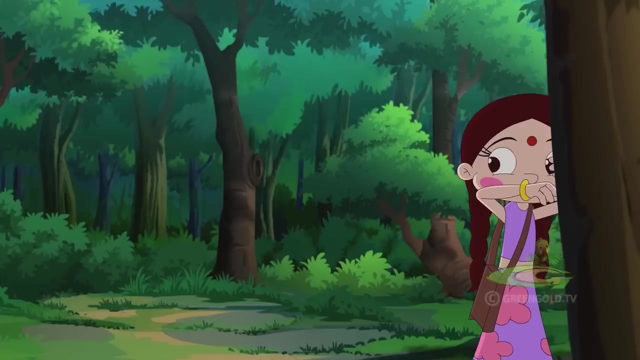 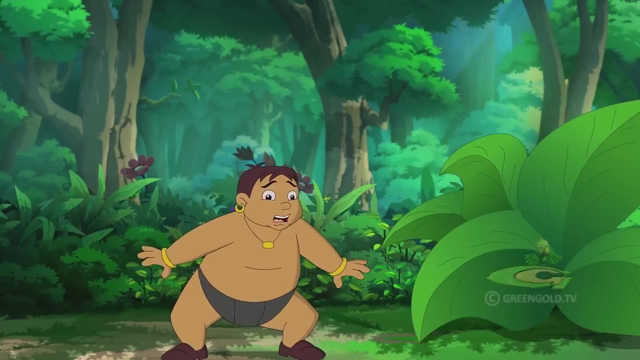 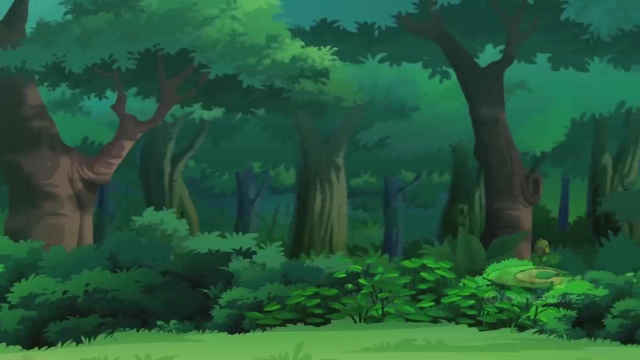 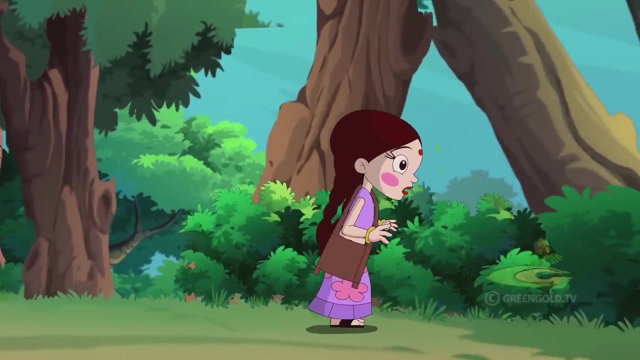 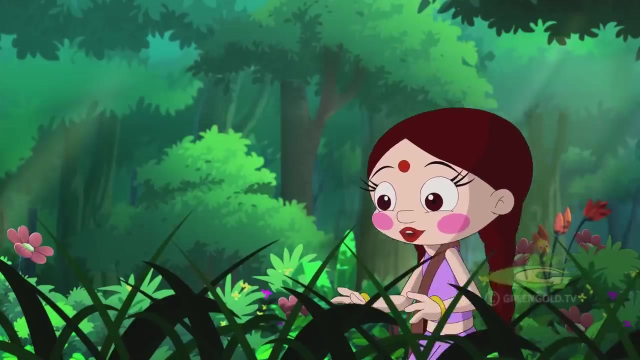 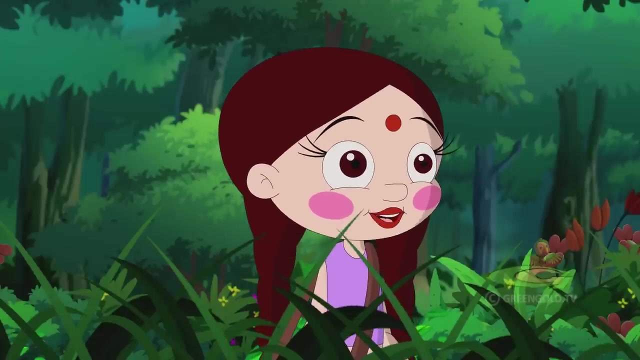 98,, 99,, 100,. are you ready now? Not as yet Ready guys, Not so fast. Huh, I'm coming now. Huh, Where is everyone hiding? I could always catch them so easily, Huh. 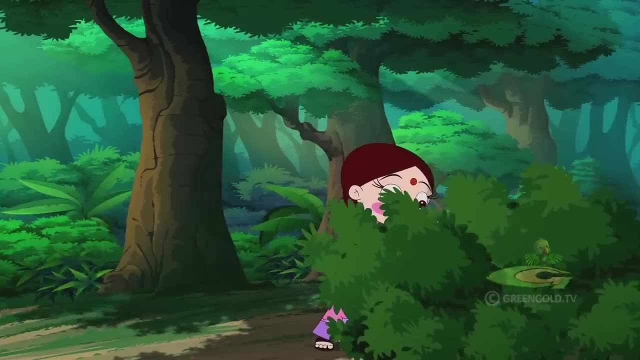 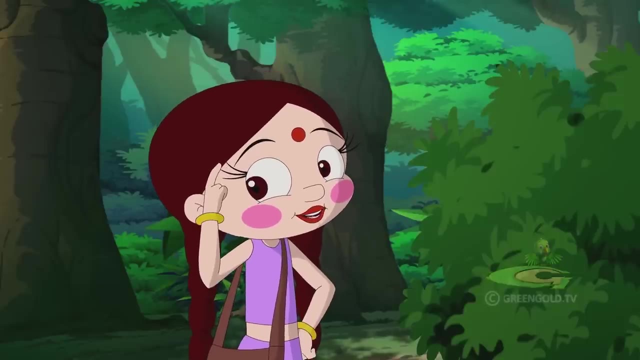 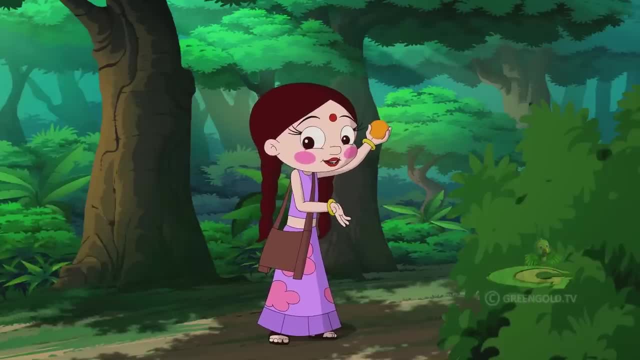 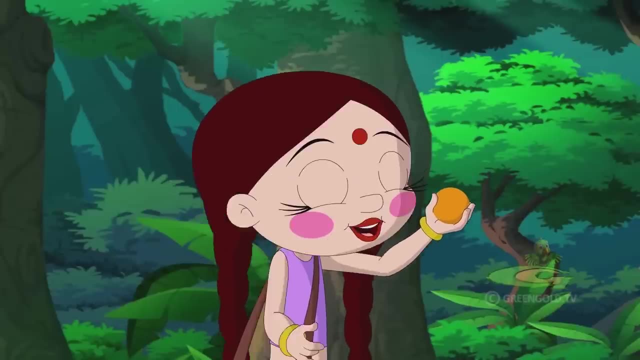 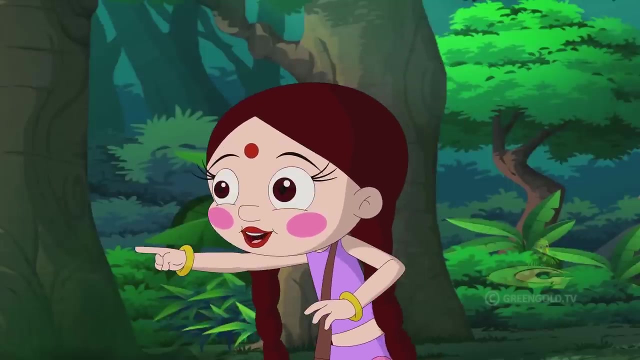 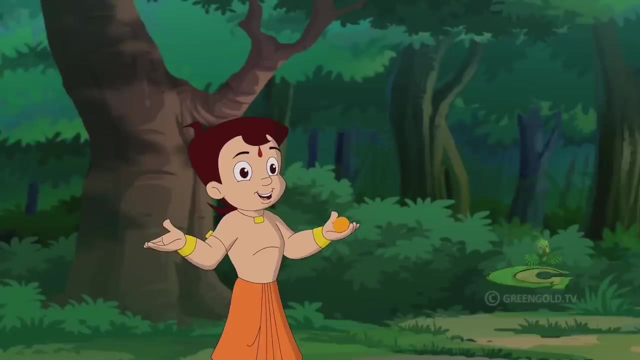 I'll catch them. Keep it clean, STAR KIT. Huh, Get closer, Stop, Stay here. Keep stands, Don't be afraid I will get you down. Anyone would do this for such a nice laddoo. I agree completely. 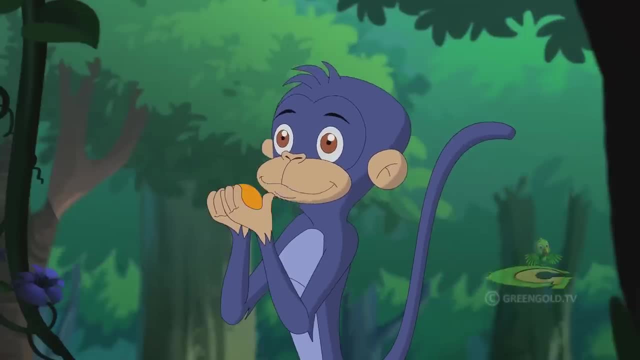 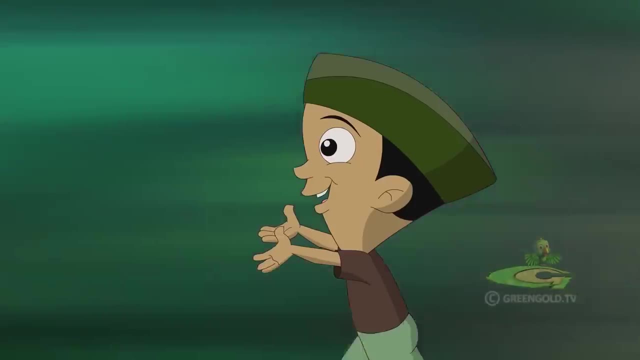 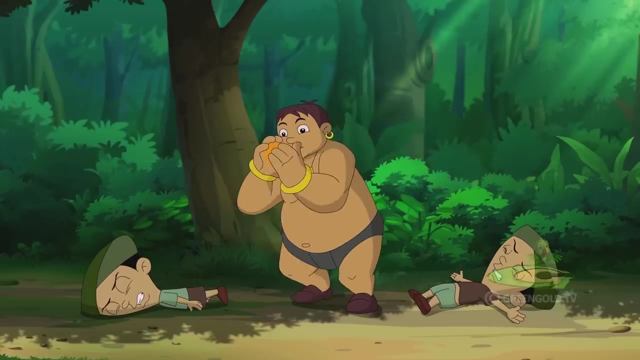 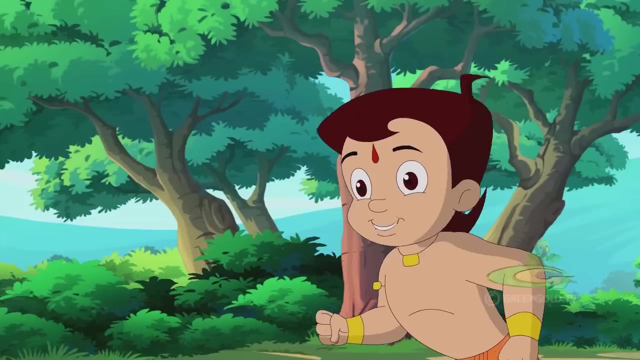 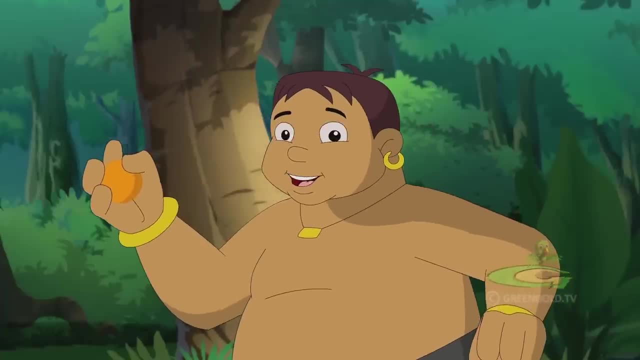 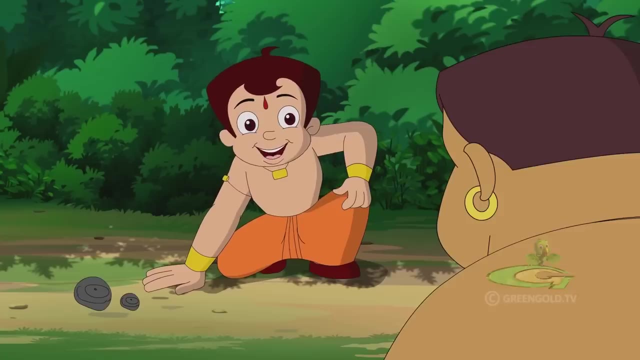 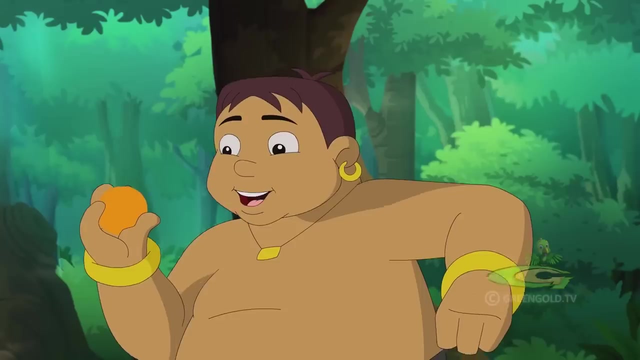 So you better admit that today is not your day. Vim, Give up now, The game is over. The game is not over yet, my friend, Because I don't give up that easily. Well, we may have just one laddoo. 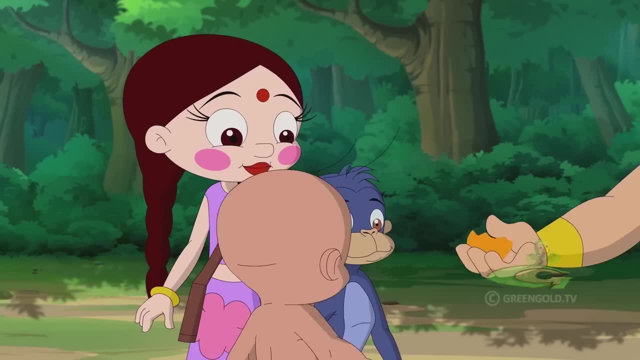 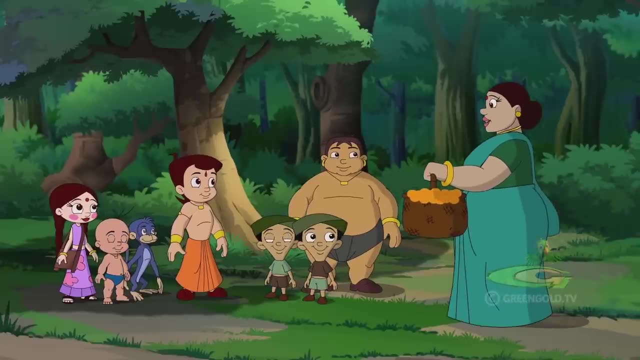 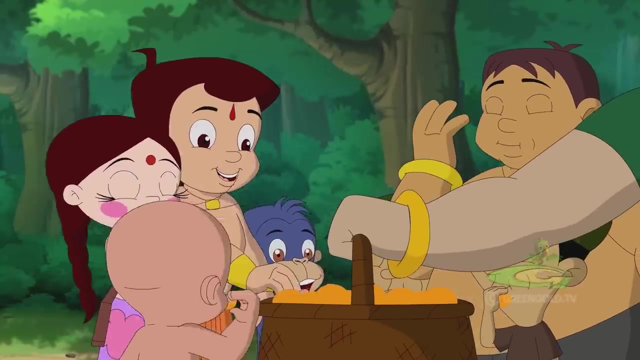 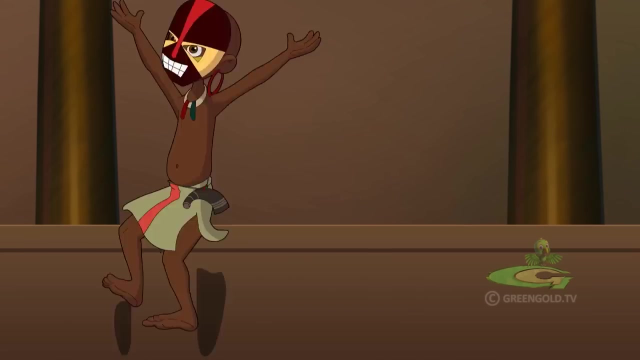 But if you agree, we all can share it. Well, kids, there can be no shortage of laddoos till your Tintun. aunty is there. Yeah, you can all have them. Oh, yeah. What nonsense is this? 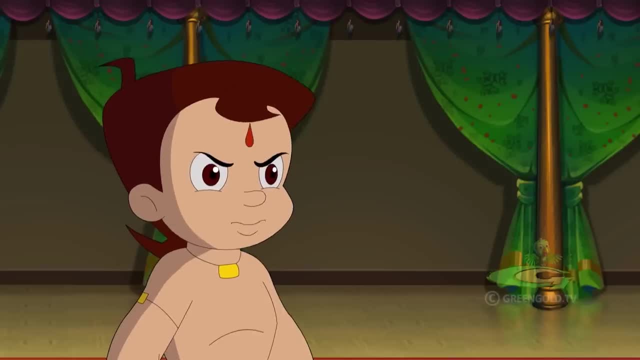 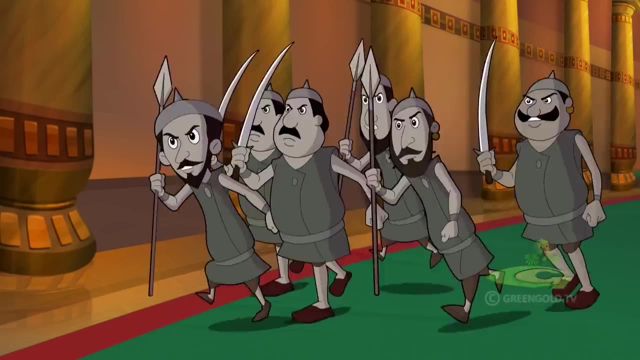 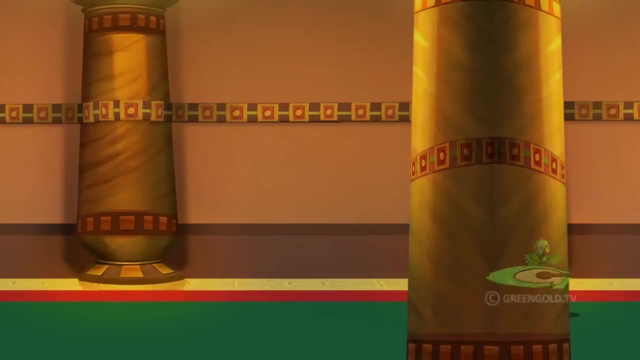 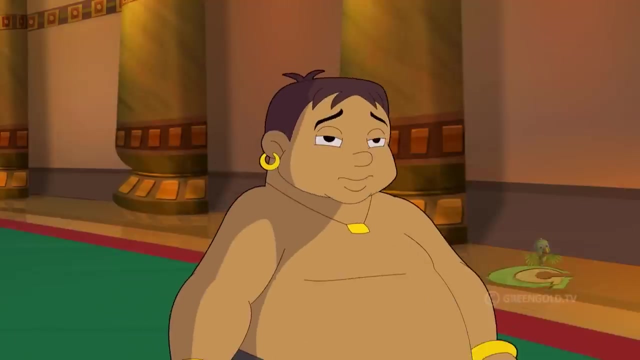 Halt, I say, You can't escape from us Guards. catch that thief, Don't let him run away. Wait, I'll catch this rascal. This thief is quite agile. Hey boss, We never knew you were so good at headbanging. 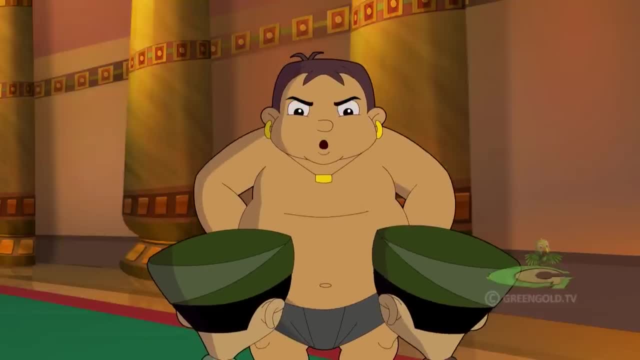 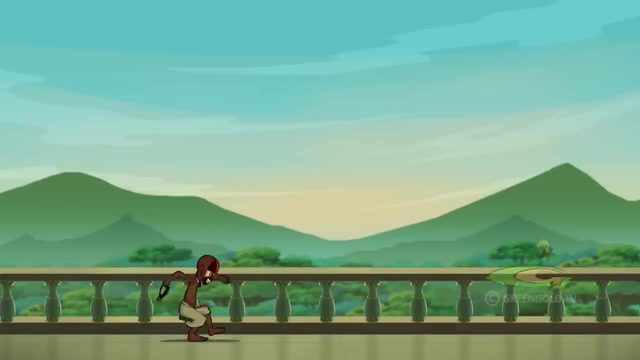 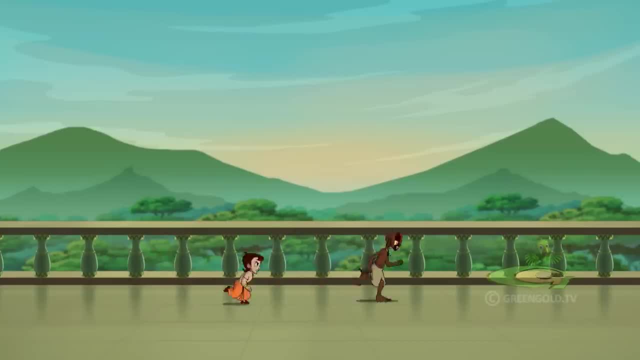 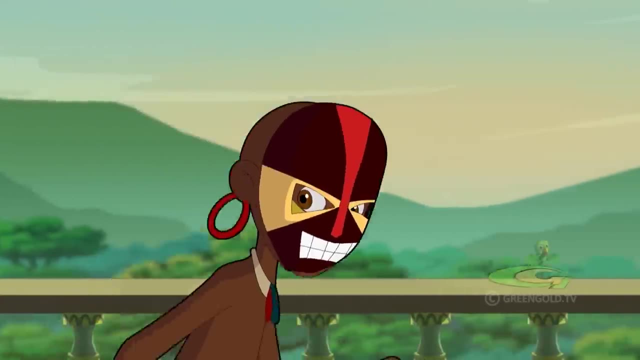 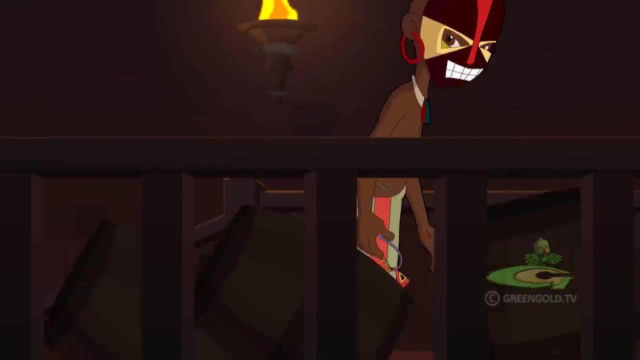 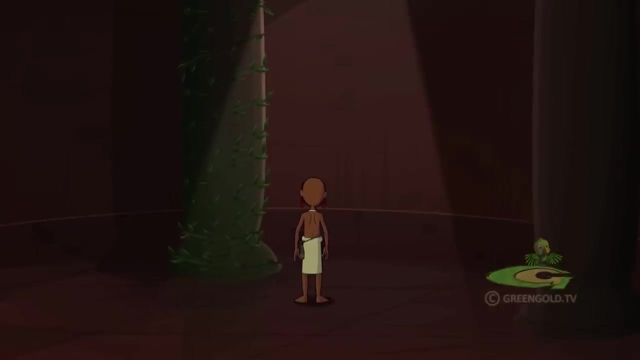 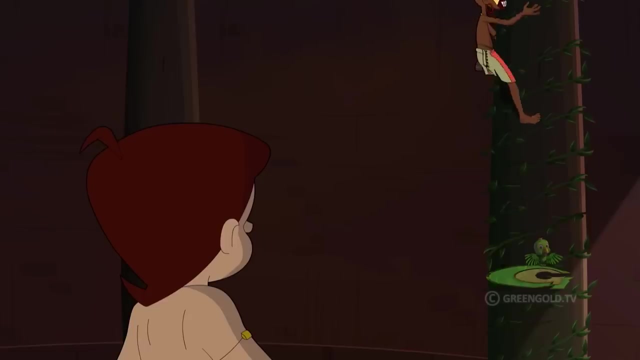 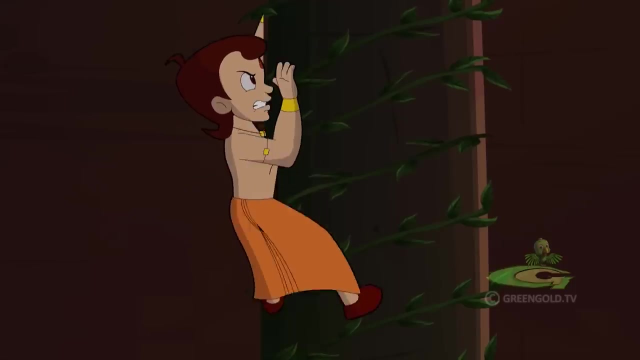 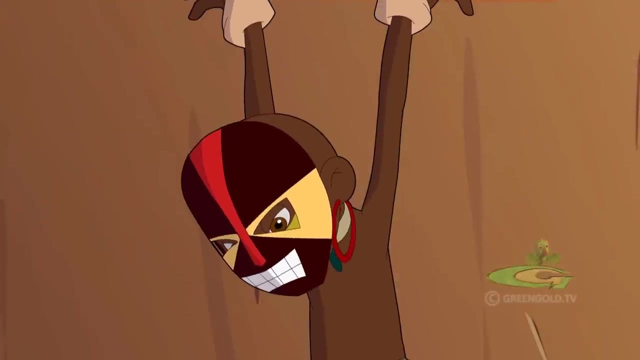 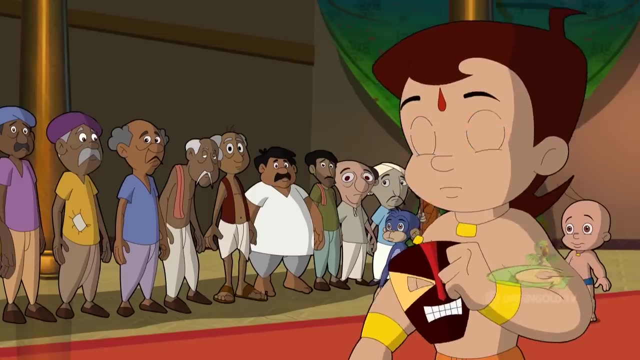 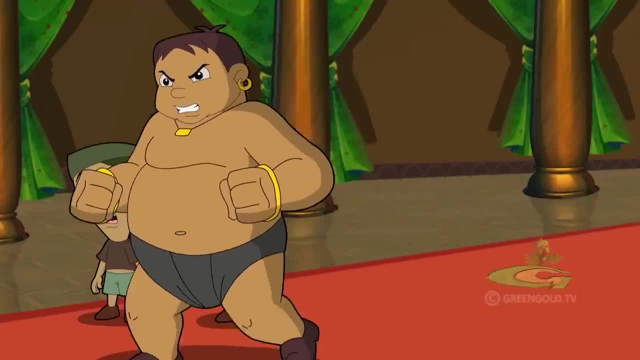 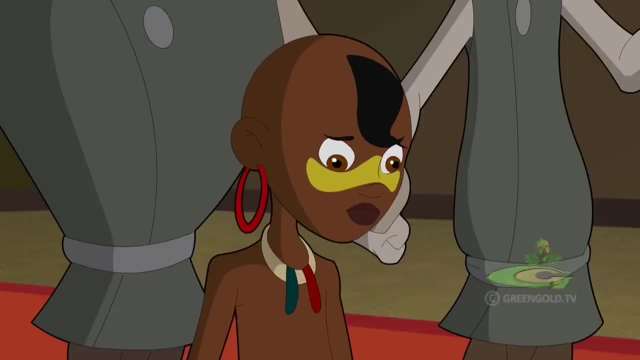 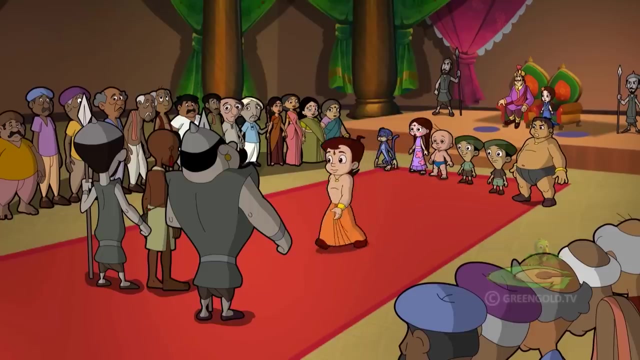 I will teach this muddy a nice lesson right now. Just wait, Hold on, Kalia. Let's first find out Why this boy attempted to steal this. I know how to make him speak. No wait, Kalia, Let me ask him. 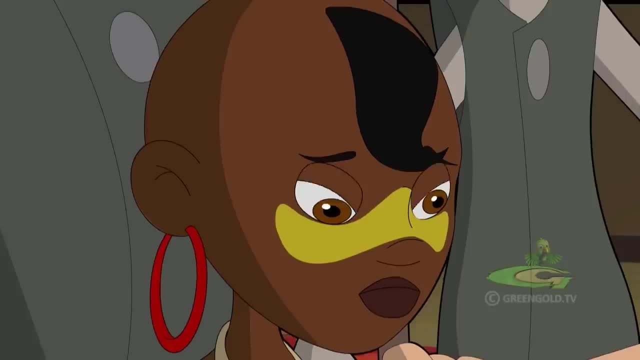 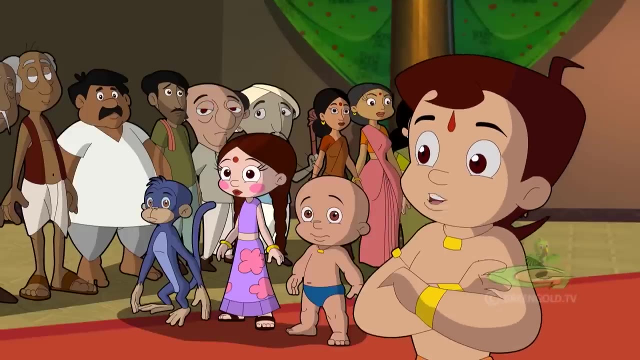 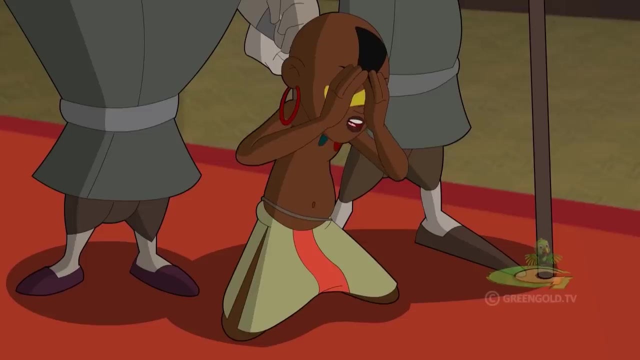 You could have easily escaped, But I know for sure you're not a robber and you're surely in some kind of trouble. Tell us everything. Maybe we can be of some help to you. What, What, What's that? What's that sound? 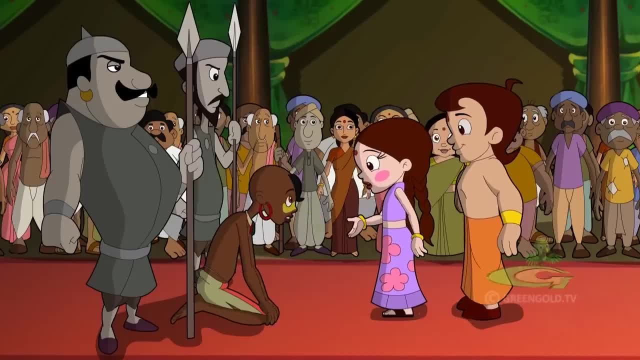 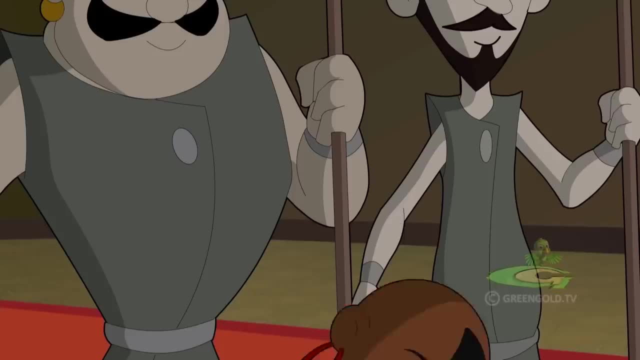 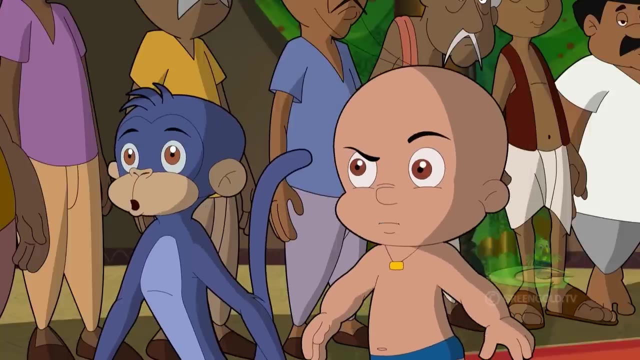 What's that? No, no, no, Don't cry. No one is your enemy out here and, believe me, all of us are going to help you. Take a look, I've come all the way here in search of this thing. This is a picture of the same amulet, Bhim. 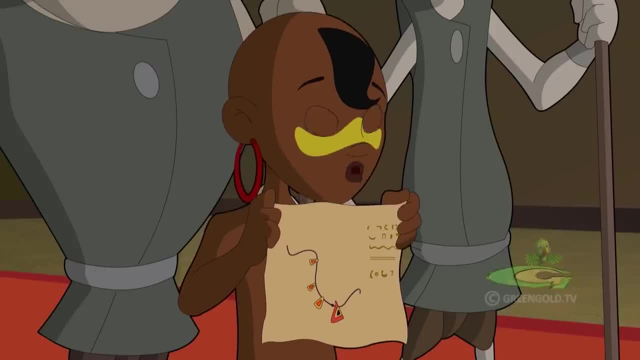 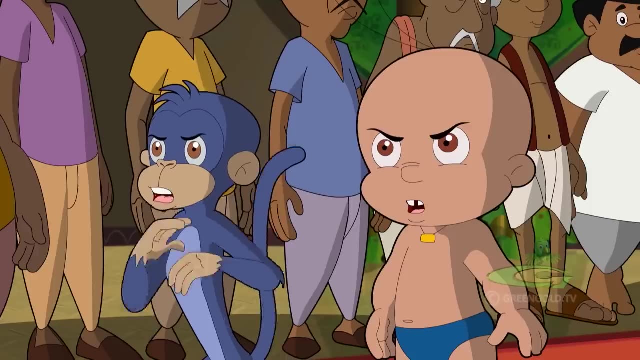 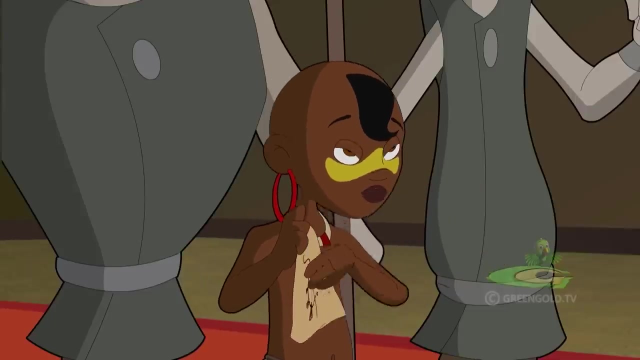 Who are you and where did you get this from? My name is Duray and my father gave me this map When a village was attacked. Huh, Who attacked your village and what for? This is not any ordinary amulet. This is one half of the most powerful amulet on earth. 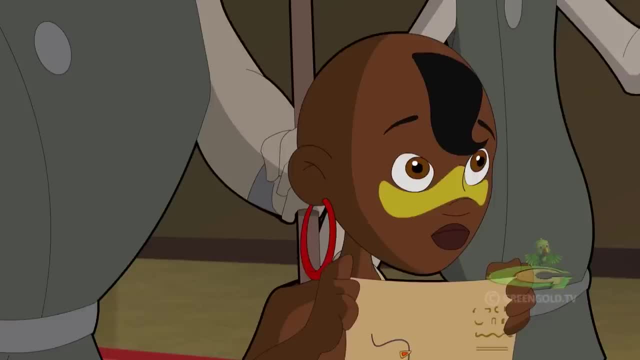 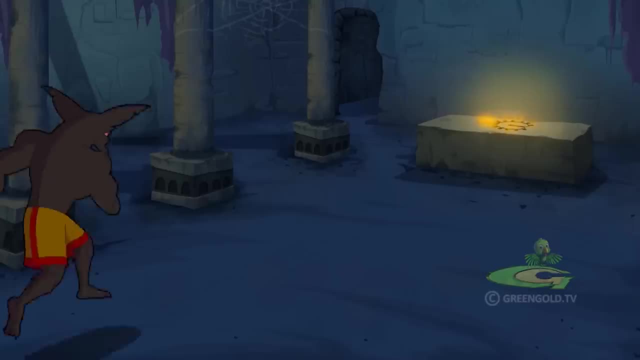 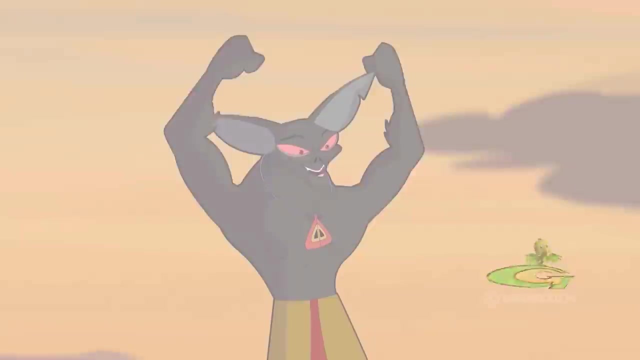 Our village has been guarding this amulet for thousands of years, But a thousand years back, a crook named Zeracus stole this amulet from our village. He misused the powers of this amulet and turned all Africans into his slaves. 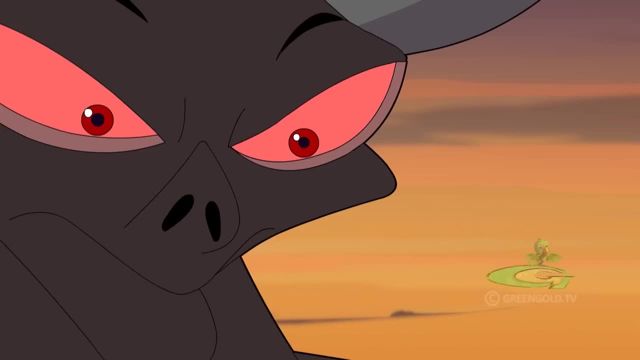 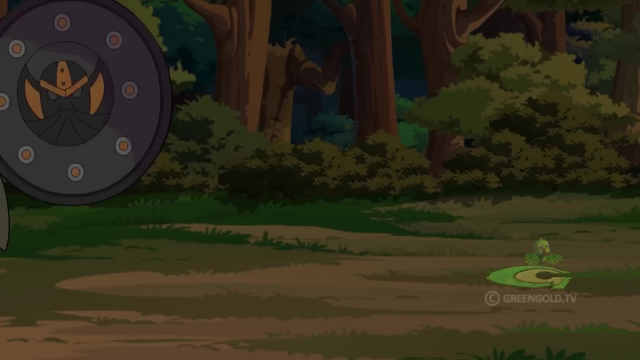 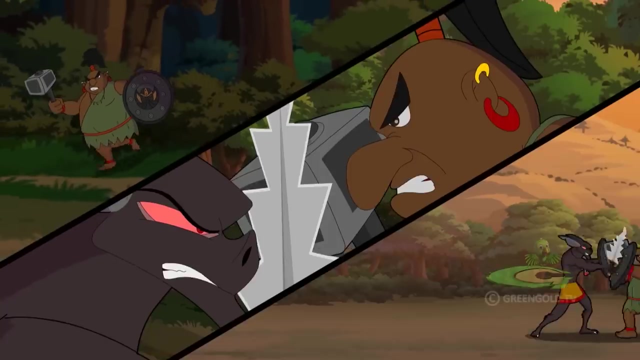 But one slave didn't accept this slavery. His name was Yuji. Yuji challenged Zeracus for a fight, and their battle went on for many days. Zeracus was much stronger and powerful than Yuji, But Yuji didn't want to fight. 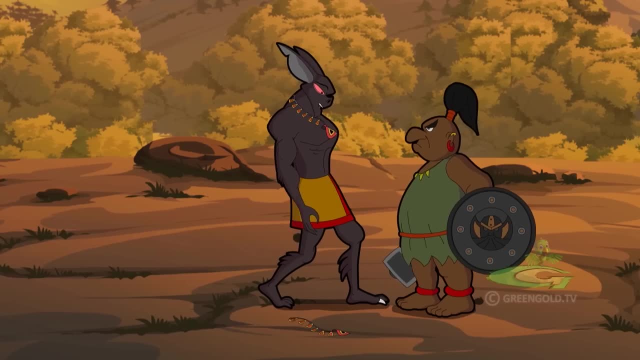 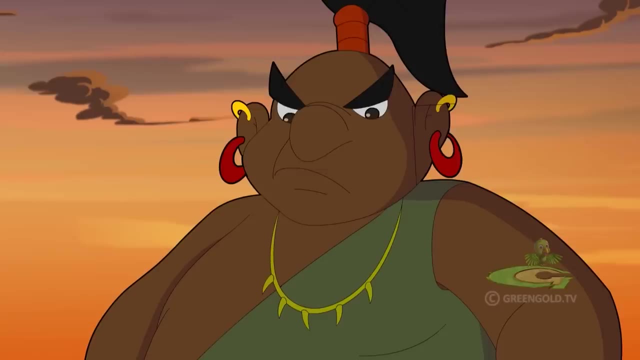 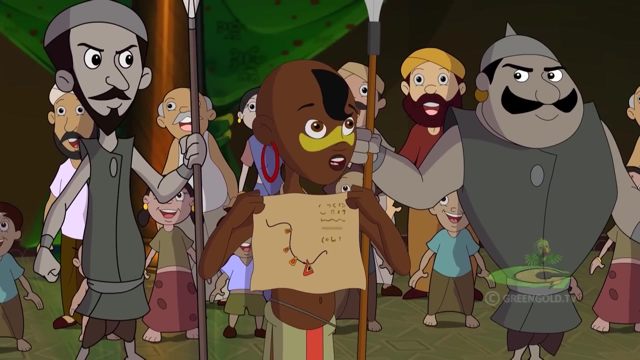 He didn't give up And in his final attack he broke the amulet into two And with a loud bang, both the halves of the amulet vanished forever. The secret of finding out and joining the parts of this amulet again has been written. 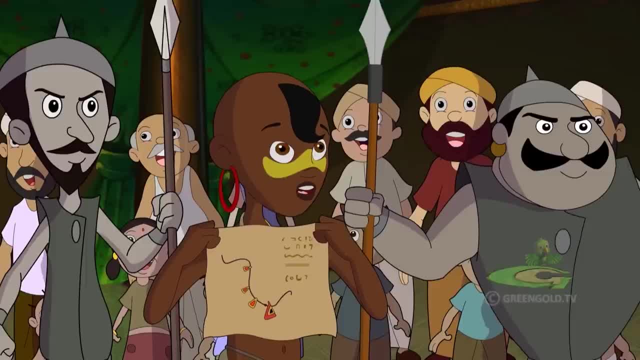 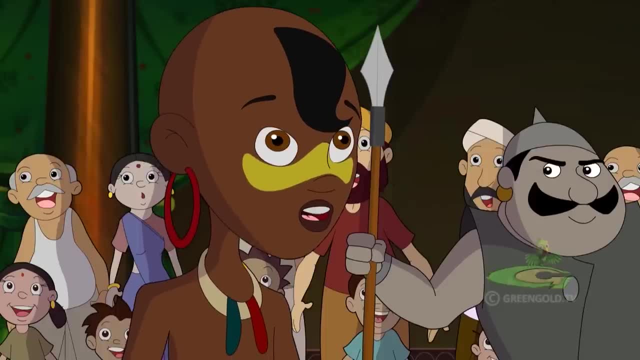 down in this map And my father used to protect this map. To get hold of this secret, Girboro attacked our village. Now, who is this Girboro? He is an evil tribal. He is a rebel. He is a rebel leader. 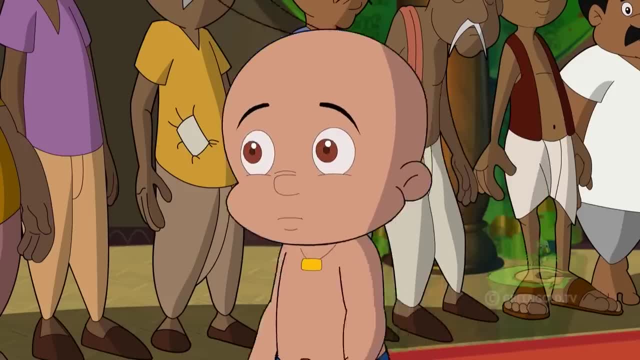 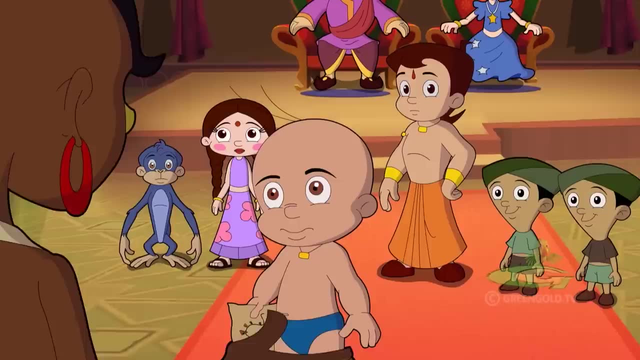 And he wants to turn the people of Africa into his slaves once again. But this is just half the map. Where is the other half of this? With my younger brother, Gano, My father tore this map into two and gave one half each to both of us. 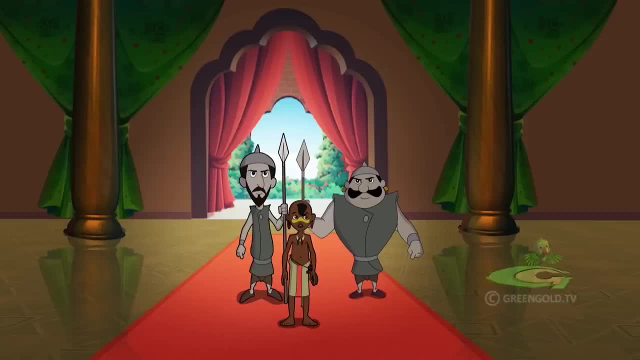 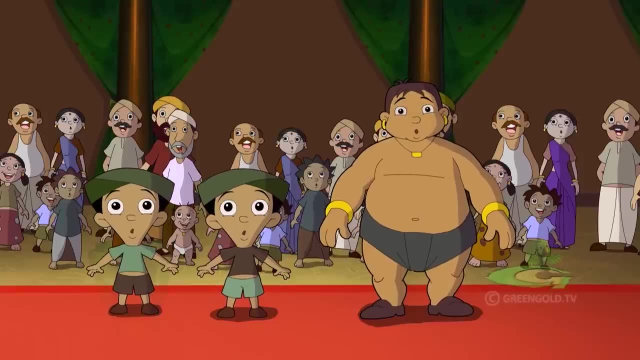 Huh. So where is your brother now? When Girboro didn't get the map anywhere in the village, he sent his soldiers chasing us in the jungle. My brother Gano, ran away inside the jungle. Girboro's soldiers also followed him into the jungle. 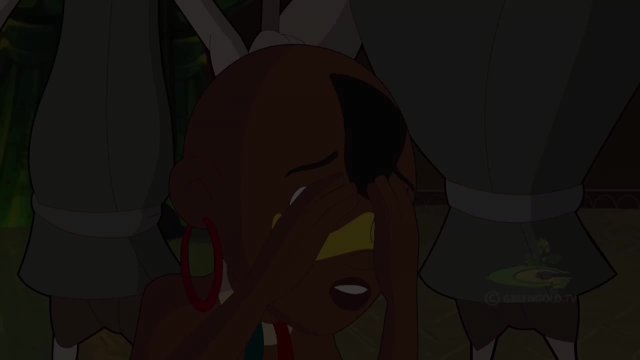 I couldn't be of any help to him. I got so, so scared. Look out there Dark clouds. This means the sun will shine and there will be rain too. Finally, there will be some rain in Dholakpur, And then we'll jump up and down in the puddles. 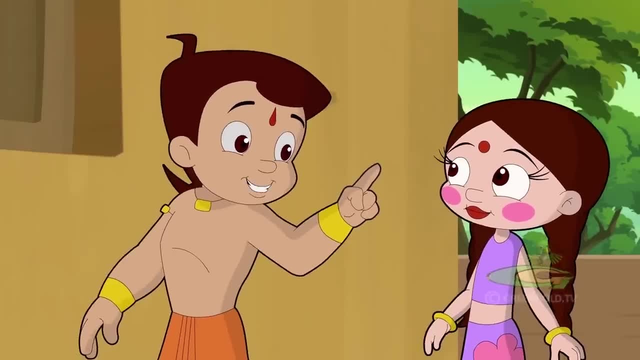 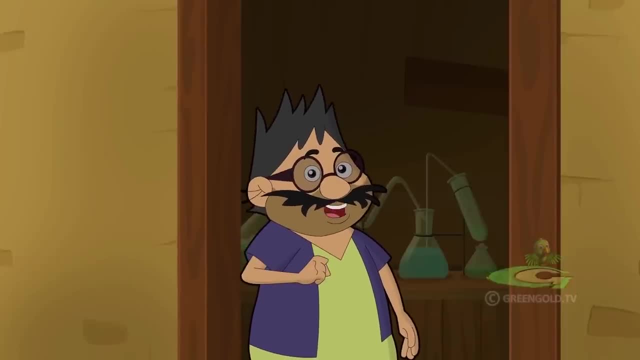 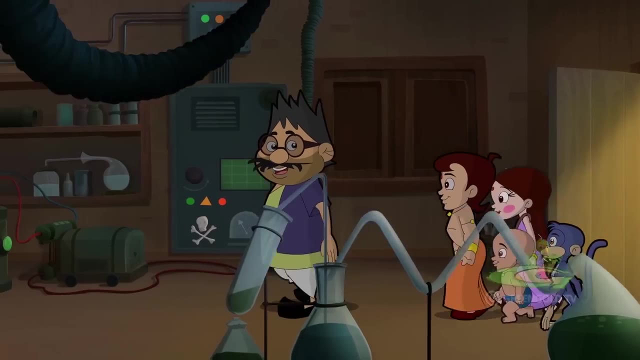